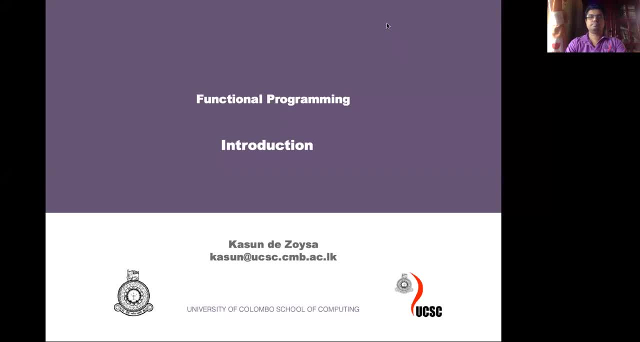 Functional programming. So in the introductory lecture today we discuss types of different programming paradigms and the difference between functional programming and other programming styles and one of the leading functional programming languages. So with that lecture we're going to start a new journey: functional programming. So I know that so far you've learned the imperative programming, and so this lecture onwards I'll teach you how to shift from typical imperative programming into the different programming styles or the paradigms. 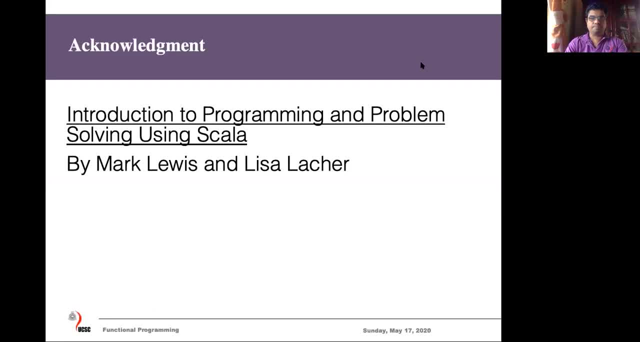 For example, functional programming. So I'll refer one book in this course: Introduction to Programming and Problem Solving Using Scala. So electronic copy of the book I have shared with you. So I recommend all of you to read the entire book. 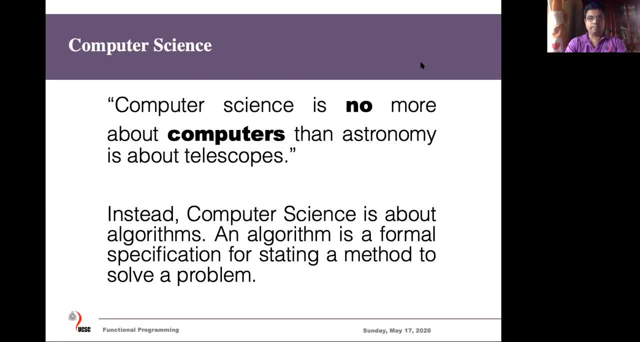 Let's start our journey. You know computer science is a very huge area right now. That teach not only computer, So computer science, teach about algorithms and the method of solving those algorithms, how to specify those algorithms and how to optimize those algorithms and so on. 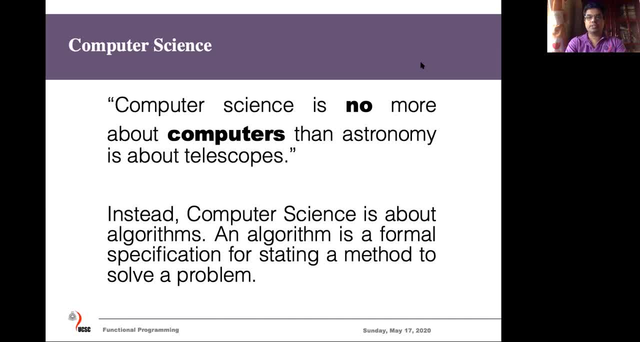 So it's similar, like when you say astronomy, So people might think it is about your school. So when you say computer science, it's not Obviously we need the computer in the computer science area. but computer science is somewhat larger area. 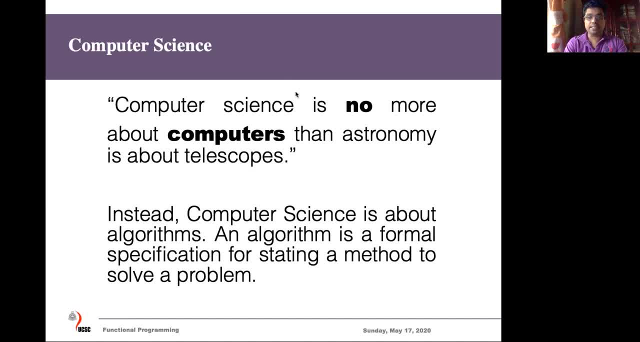 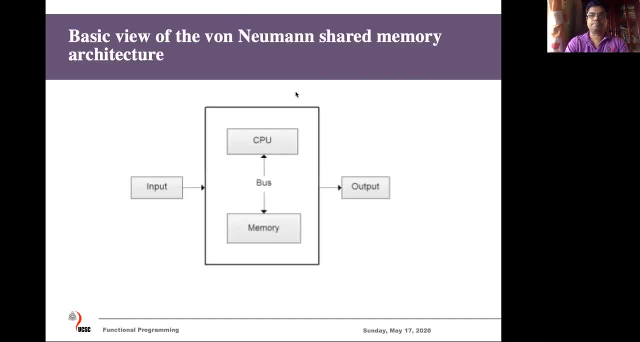 So mainly that is all about solving problems by using algorithms. When we come back to the computer, you know basically computer has inputs and outputs. Then there is a device called computer where it takes that input, do front processing and create an output. 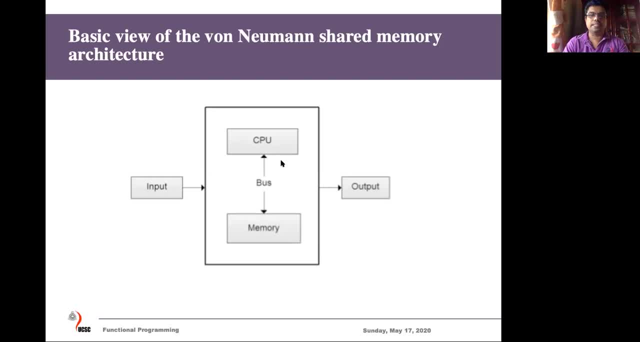 So the result will be stored in the memory or some other storage device And the processing happens in the CPU, So in the computer, in basically some device which takes some input and creates some output. So the functional programming is similar to that We will discuss in a minute. 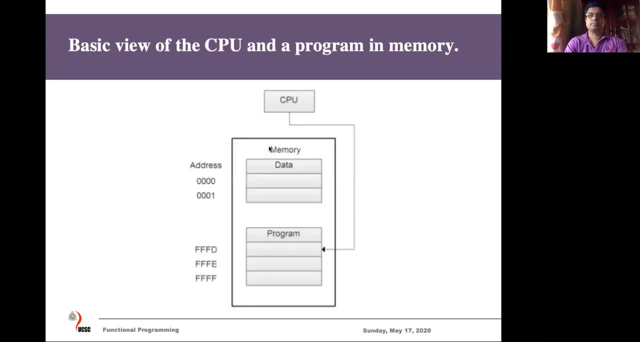 When you take the CPU in the computer you know we take the data and programs. Special programs call it as instructions. We store those instructions in the memory Plus the data in the memory CPU fetch the instruction. Based on the instruction, they fetch the data. 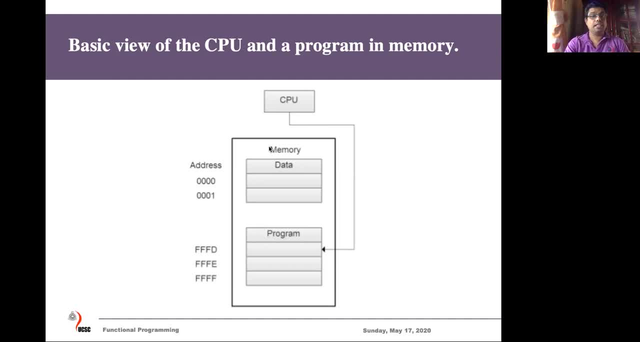 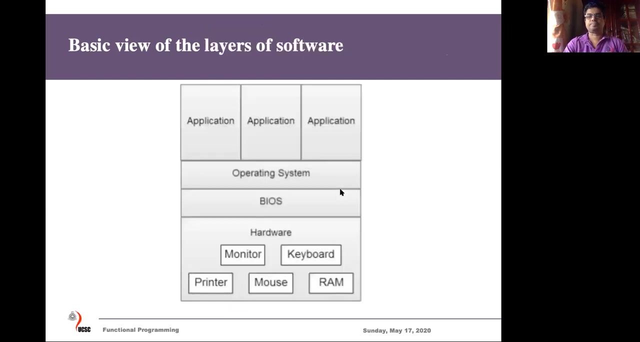 And they process the data And store the results again in the memory. So when computing memory is kind of, you know, very important place Where we store data plus instructions, You know, in the basic computer structure in the low level what we have is hardware. 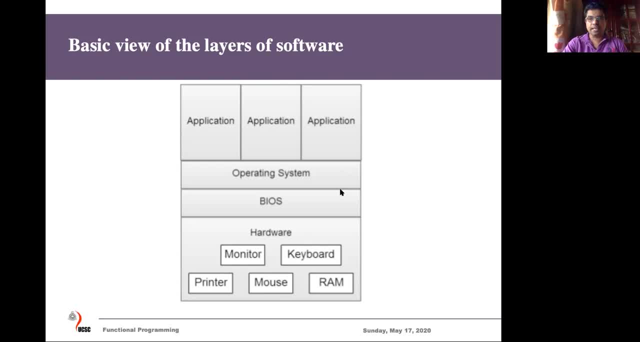 So on top of the hardware we have some software layer. We call it as basic input-output system. So using that basic input-output systems, So people have implemented some kind of software. We call it as operating systems. So then we write applications on top of the operating systems. 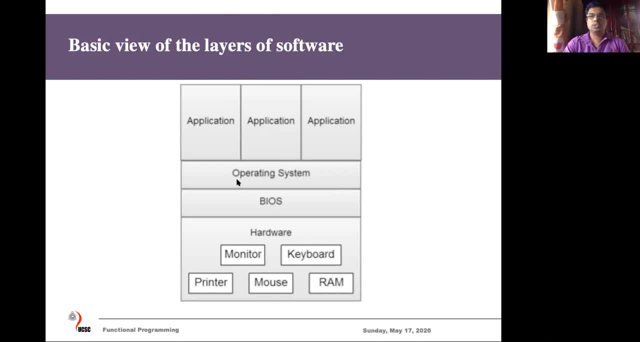 Our applications usually talk to the operating systems And it converts it, pass that instruction to the basic output, Basic input-output system towards the hardware To perform our action. So, as an application, they may not see the real hardware, They see what we call it as abstraction. 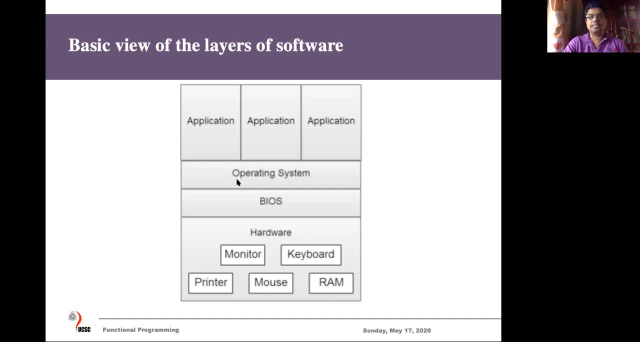 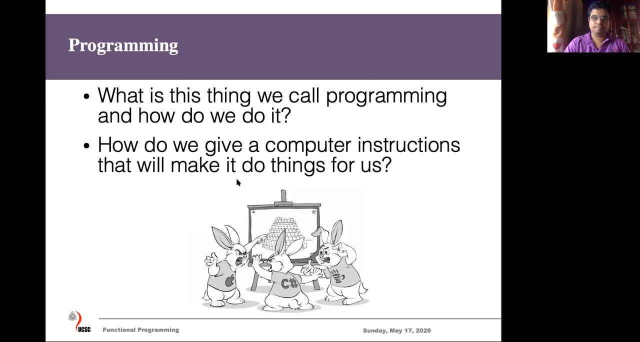 Some kind of abstracted layer provided by the operating system to the application. So by doing that, we So by doing that, we simplify implementing the application. Programming is something like giving instruction to the computer to perform some set of actions. 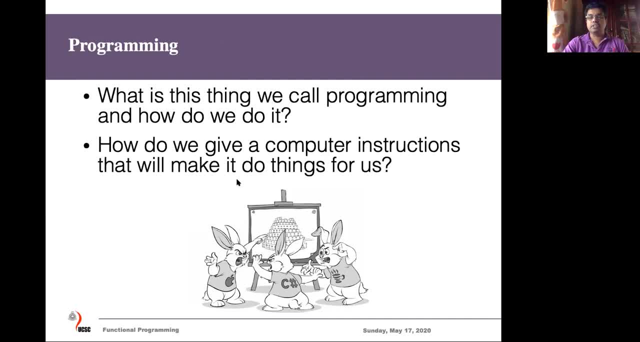 So we can give instructions in abstract manner On top of application layer Or we can give instructions in the normal layers. So programming is somewhat we call it as giving instructions to the computer to do or to perform meaningful action. If you do that instructions. 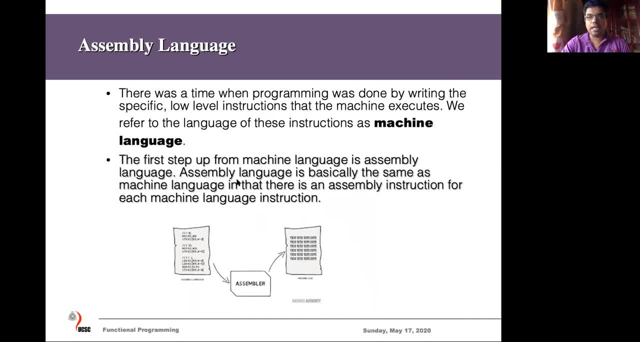 Or if you, If we give that instructions in the lower layer, So we call it as machine code In the machine code Basically pass the lower level instructions Usually once it goes to the machine. At the initial stage of computing we did that. 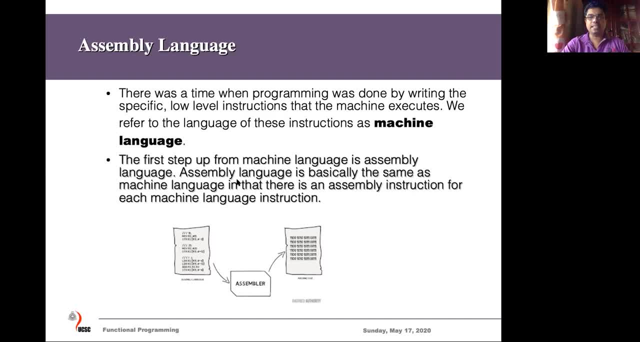 So passing that lower level instruction is very inconvenient for humans, Even though it's convenient for machine. So we need to have some abstraction. So at initially, The computer scientists have developed some kind of program. Well, it has assembler. 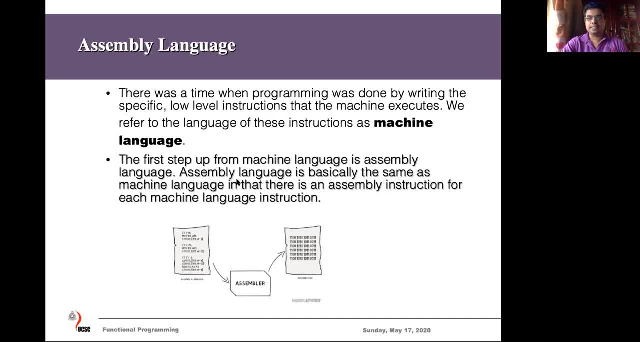 All of our assembler is to convert Some meaningful Instructions To the machine, To the code, Machine code. So in other words, Some people have developed a program that can identify Or that can understand some codes Such as add. 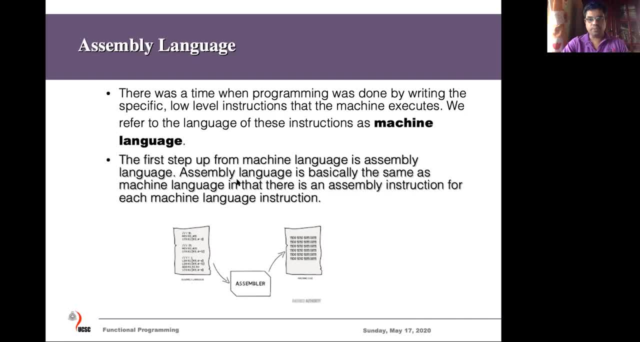 Subtraction Move, Jump, Like that three letter code. So this three letter code can be converted into the corresponding machine code of the computer. So then people can write a program using this three letter code And give that file to the compiler. 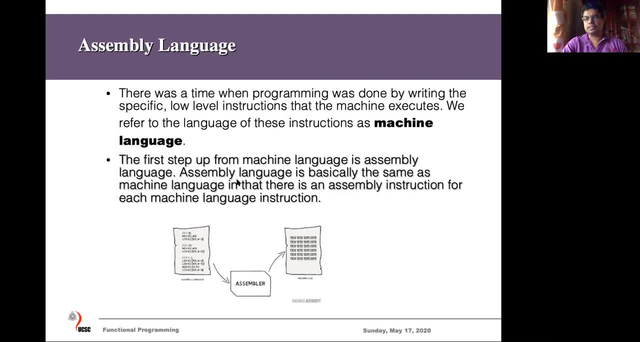 What you call it Assembler, That convert it to a machine instruction. So then We get a flexibility To writing the code in little high level Language. So we call it as assembly language. So that's how the programming starts. 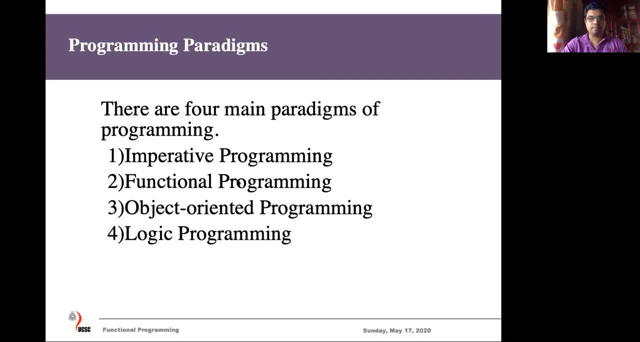 So after that, Computer scientists have think about Developing efficient methods Or the efficient way of abstraction To handle Programming. So they have developed different levels of Programming Language. That's what we call it as programming languages Idea. 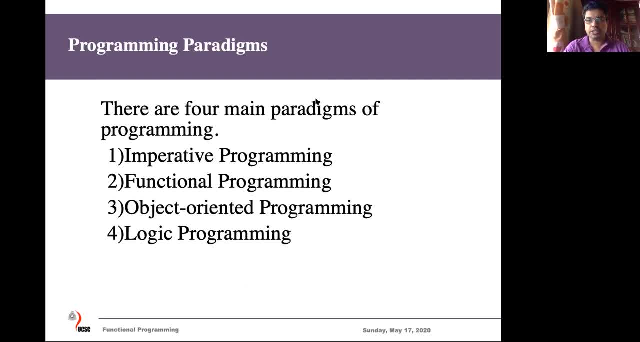 Or the concept of all those programming languages are to give instructions To the machines In the human readable Efficient Formats Or human readable efficient methods. So history start from the assembler To right now. People have developed thousands of different programming languages. 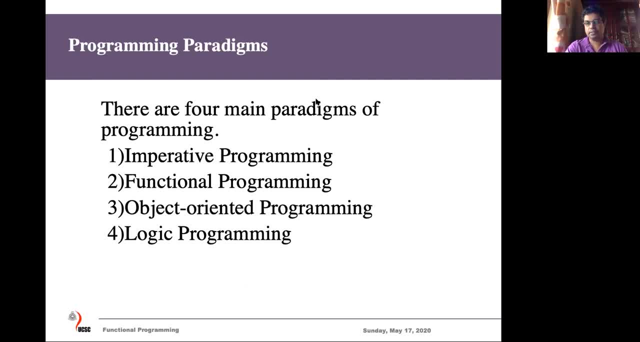 To do programming. Some people Kind of restricted yourself To a single programming language, So like You might Prefer some programming language you learn first, But as a programmer You should be able to Handle any kind of programming language. 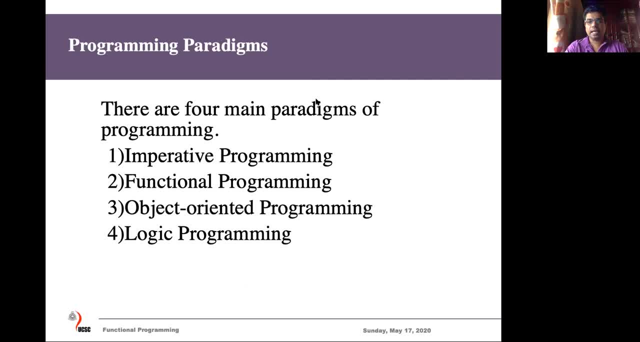 So if you learn the concept of programming And different- what you call it as different- programming paradigms, So after that You should be capable of learning any programming language In short Period of time, So In your university life. 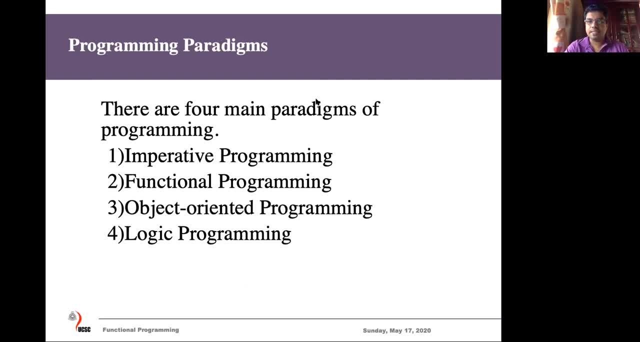 You have started programming with What you call it as imperative programming, So we give instruction there one after other, And then you learn little bit of, I guess, Object oriented programming, And now you are learning functional programming. So there are some other paradigms for logical programming as well. 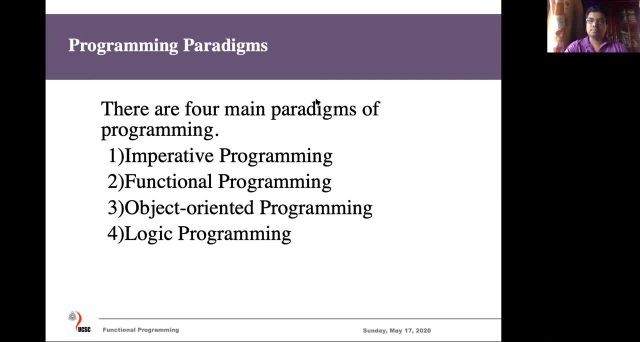 Most of the programming languages In the computer Kind of imperative Programming. So Whatever programming language used at the low level, It's converted into the machine code. Machine code Execute those instructions one after other. It is like a sequence. 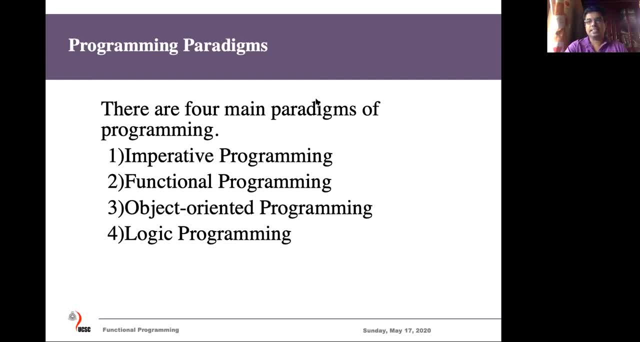 It's imperative programming Basically test the system How to do that. Actually, computers are machines In low level. We need to tell the computer How to do these things. So if you want to, actually If you want to add two numbers in computer, 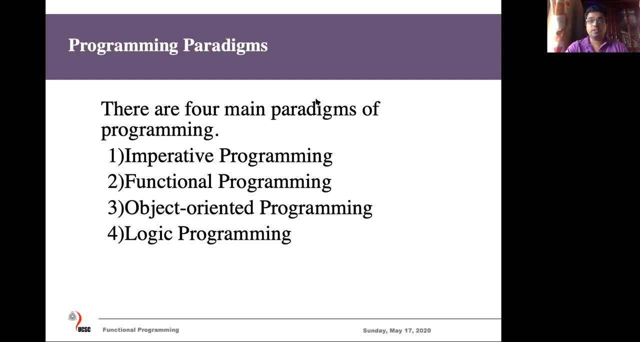 So let's say we use assembly. So first of all we have to load these two numbers From the computer memory to a temporary storage device for registers- Using instruction for me- And then we need to execute assembly code And the result will be saved in the different register. 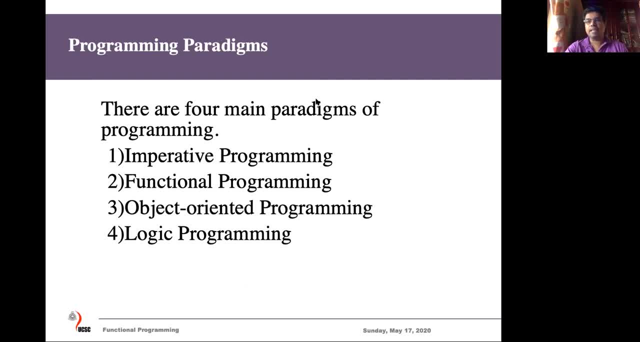 So then we have to Move that From that register back to the memory, to storage. So all those things we have to tell, Move two numbers. Move first number, Second number, Add those two, Move the result back to the memory. 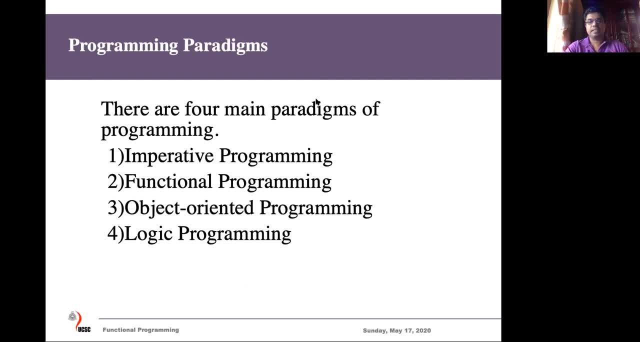 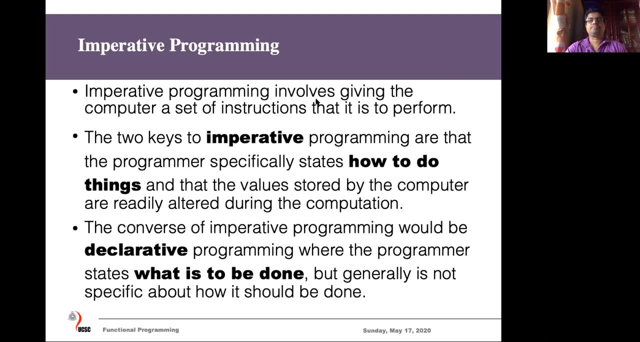 Everything we have to tell the system one by one. So that is what we call it as Imperative programming. Imperative programming Programmer specifically states How to do things Actually in the computer we need to do so, But people have different programming languages. 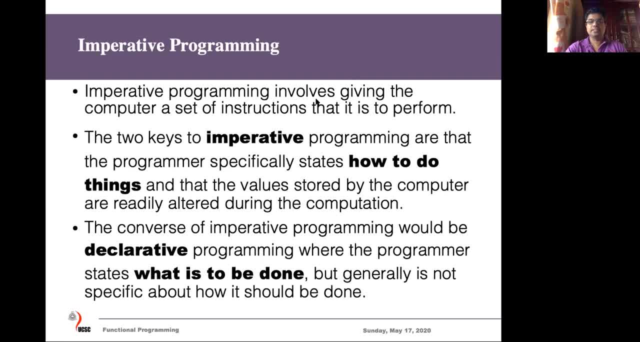 All it has declarative programming language, So in those language we don't need to tell the computer how to do things. We tell the computer what is to be done, Then computer decide how to do that. So that is simple. 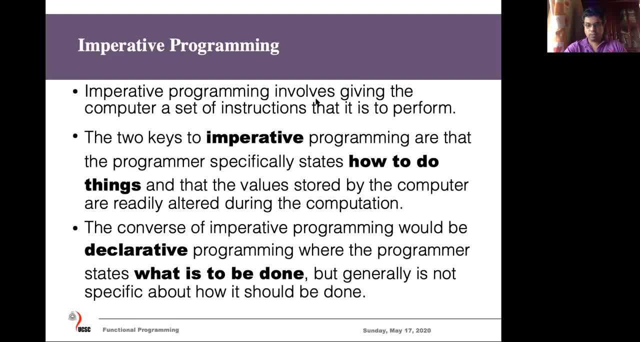 For some To source some functions So programmers Can tell the system. This is what I want. This is what is to be done. Then programming language, convert those instruction To the imperative code And tell the computer what, How to do things. 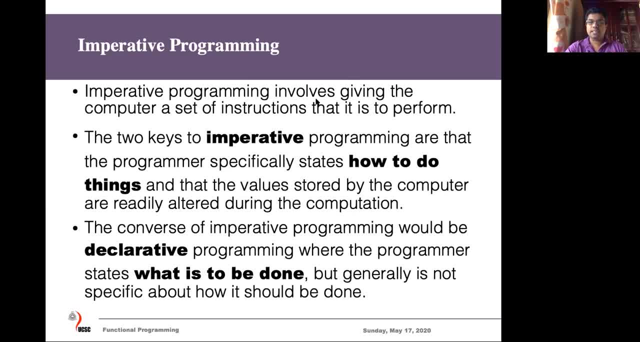 So programmer it is what is to be done, And compiler tells What is to Be done, what is how to do things. so most of the programming language in the world we can basically categorize itself into these two categories: imperative or declarative. 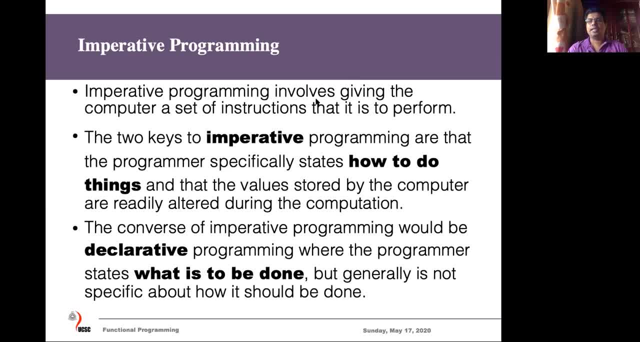 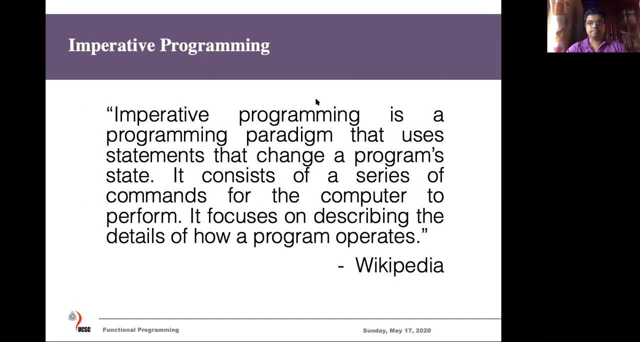 so I think so far you have learned kind of imperative program. so this is the course where you're going to learn declarative programming. so one of the declarative programming method is functional programming, right? so Wikipedia defined imperative programming as this. it says imperative programming is a. 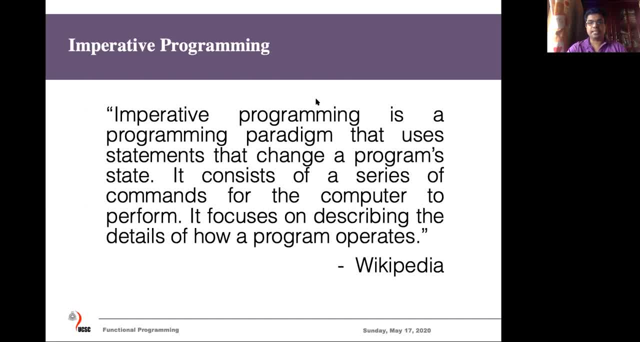 programming paradigm that uses statements that change a program states. it consists of series of commands of computer to perform. it focuses on describing the details of how a pro program operates. so instruction will operate or execute one after other and the result of these executions store in the states, different states in the memory and finally it arrives the. 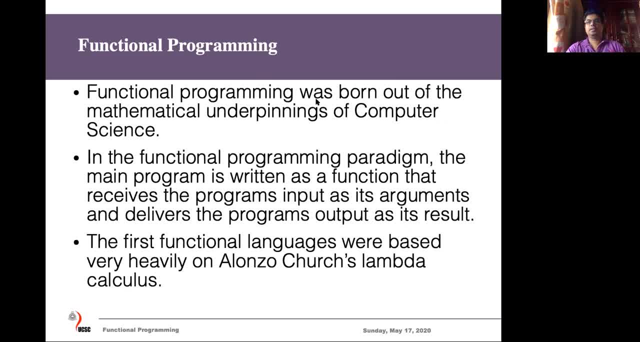 results. opposite of that paradigm is functional programming. so functional programming follows the imperative programming state. functional programming bones in very early stage of computer science due to a kind of mathematical language developed by some researchers. this language they call it as a lambda catalyst, so they use a letter lambda to define these mathematical functions. or 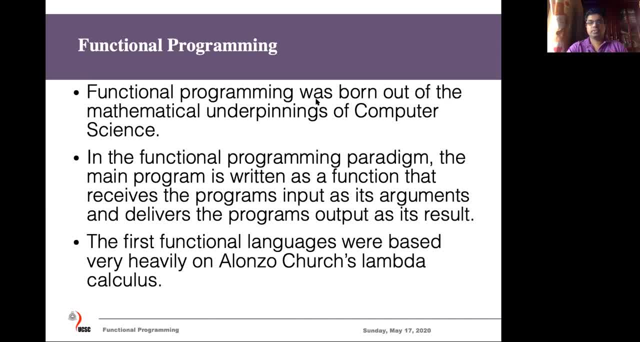 the methods. so it started with computer science somewhere around 1930- 1940 period, so at the beginning of computing or computer science or computers somewhere in 60s. so people knew about functional program but imperative programming got popular like see. but when comes to this cloud computing era right now with 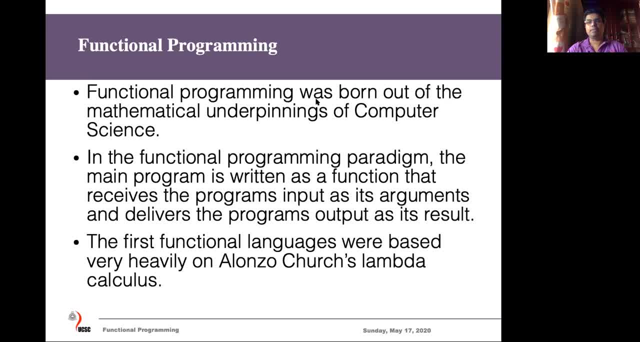 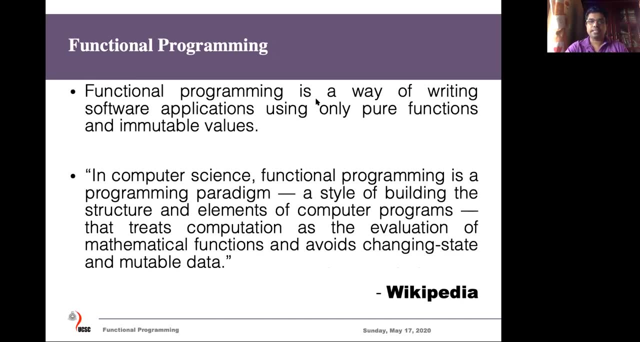 different micro services and huge programming developments. people now thinking back to the early days of computer science and computer science were able to use their own functional programming and I think I'm saying functional programming, languages, functional programming. Wikipedia says functional programming is the way of writing software application only using 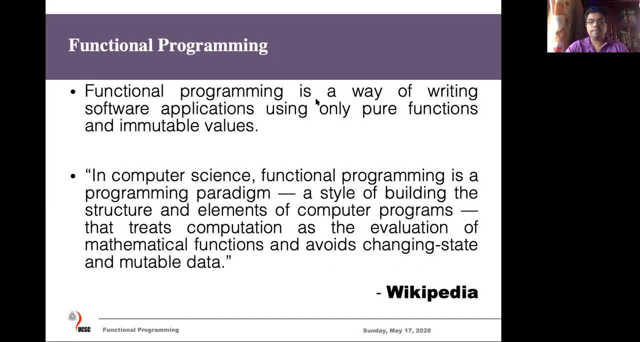 pure functions. the main value of the main, main main feature of the pure function is its immutable values in the functional programming we develop of what we call it as functions so which takes the inputs and outputs, so for same inputs, those functions always creates same output. so there are kind of evaluation of those mathematical 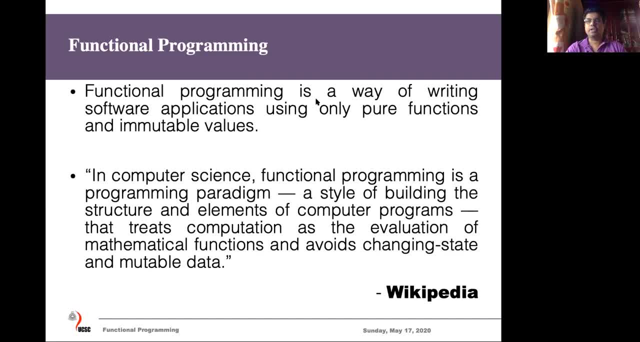 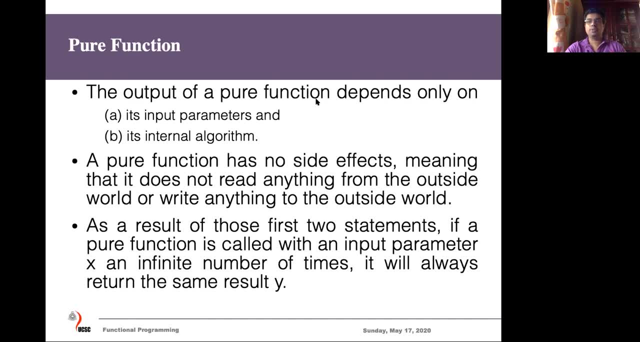 functions basically may not have any side effects. so if you want to build a pure function and programming applications, we need to divide our problem into a small set of what we call pure functions. so there are different type of functions we will learn. so in basic building block of functional programming is the pure function. 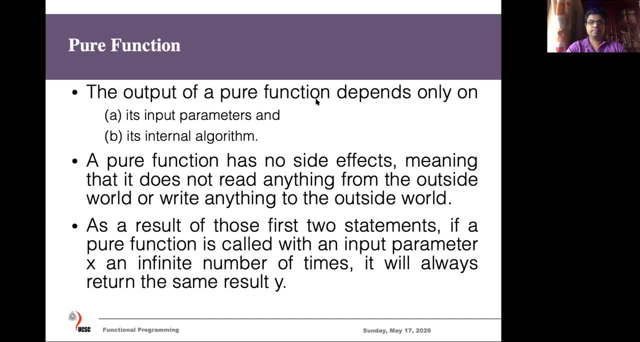 pure function has no side effects. as i said, it means does not really anything from the outside world or it does not write to anything to the outside world. like states, they take some inputs at the beginning of the functions a and they return some outputs. that's it. if you call this function x number of times or less, they produce the same result. they. 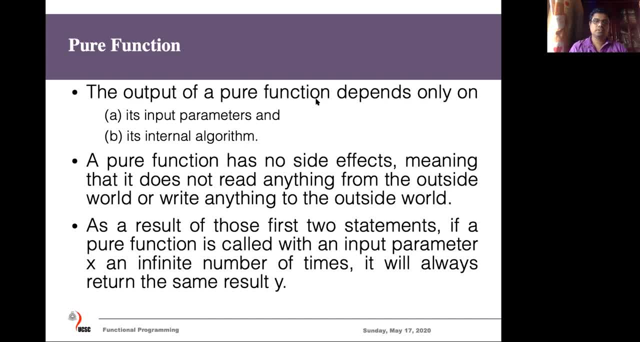 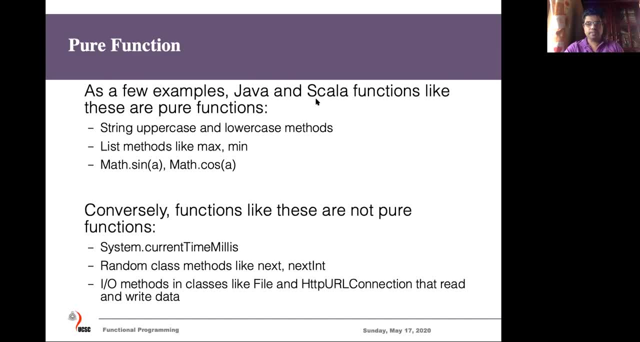 say why. so you know to understand that we need to. we can think about some pure functions and kind of other functions. so let's take function like sine function in the mathematical libraries in any programming language. when you call that sine function, sine a, with million times, the result is same, you know. 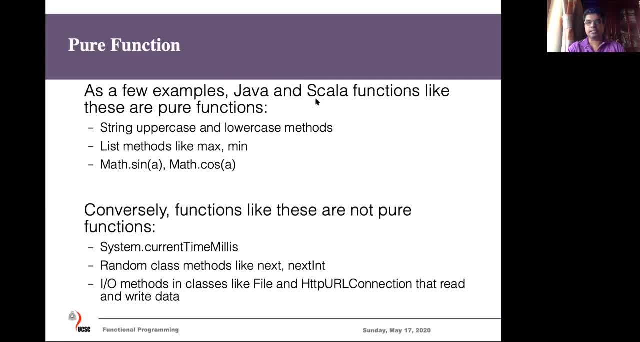 so we have given set of arrays, let's say elements, numbers, and we call maximum function max value from this list of elements. so if you call that maximum function with this input, array it from infinite of time. all the times you produce same output to the same input. yes, 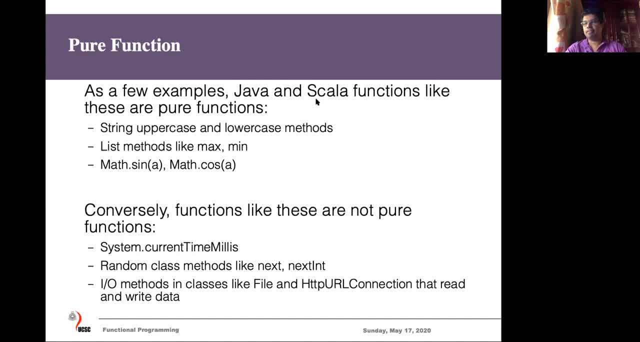 so those type of functions, like maximum, minimum mathematical functions, they are pure functions. if your functions only take inputs and produce some outputs, if you call this function million times or any number of times, it create the same output to the same input. so when you think about some function, like in the system classes of programming language, 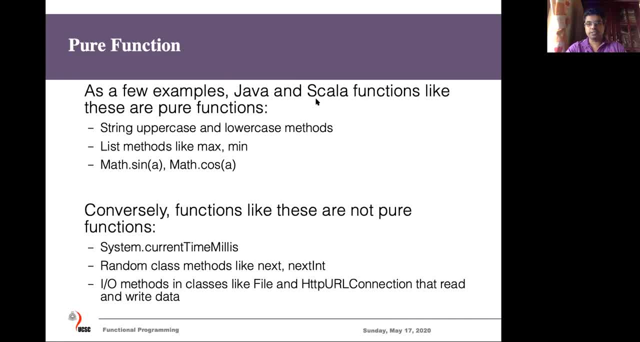 like current time functions. so when you call that function the result is the same function. the result is different from time to time. maybe in the random class in any programming language there are some functions called next it. so when you call next it, return random value next time. 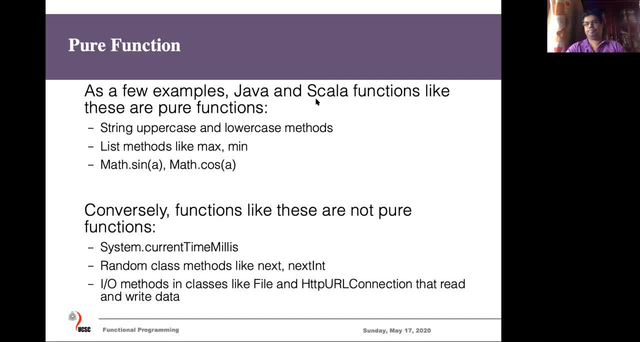 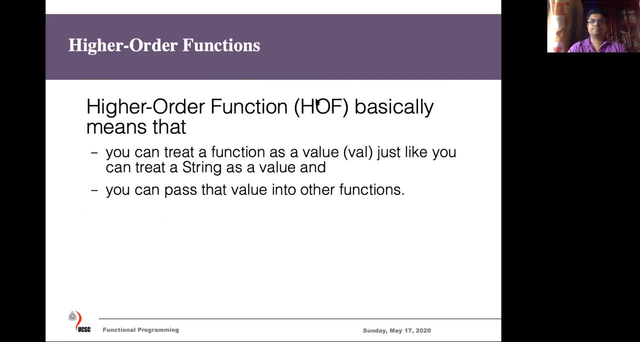 when you call next, it return a different random value. so such functions are not pure functions. then in functional programming you might learn some function called higher order functions, or some people call them as lambda functions. higher order functions are the functions which can handle like variables. so you know, when you write a function or in the methods, maybe you 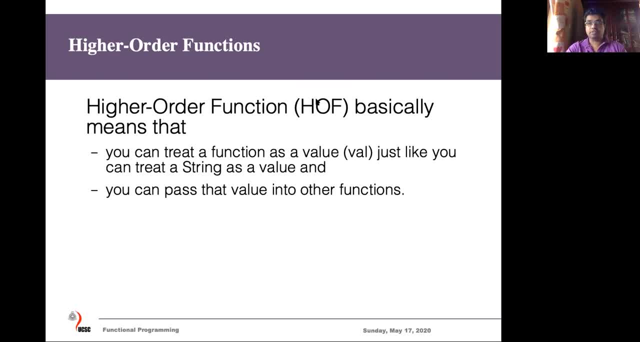 learn about method or functions in first year. so you can pass values to that. it call it as input parameters. so those input values most of the times are delta, so like integers, strings and so on. so similarly we can pass functions into the functions. we can pass some functions as: 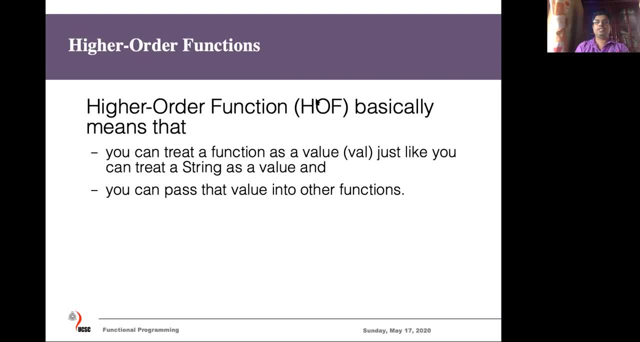 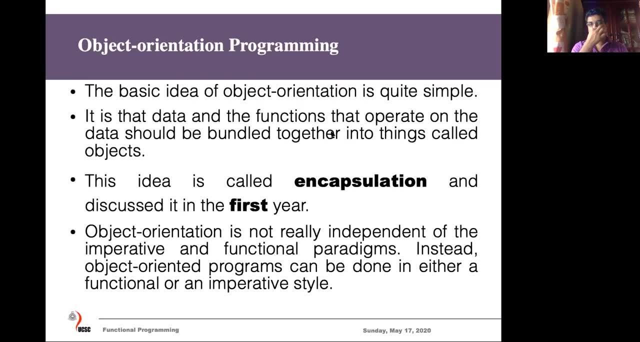 data to some other functions. so when you do that, we call these functions higher order functions. so in this course we will learn how to write pure functions, how to write recursive functions, how to write high order functions and how do you combine those functions together and so on. when you 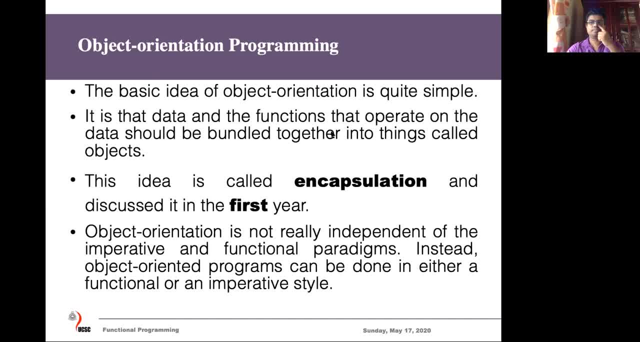 move. so it's all about functional programming language. so i think you have already learned object-oriented programming language. so object-oriented, different times of abstraction, so you can use it in different ways. you can use it in different ways. you can use it in different ways- develop by the people to do efficient programming. so in the object-oriented 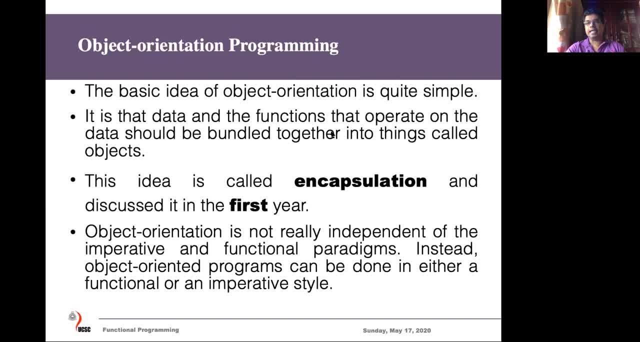 abstraction. so we encapsulate data and the methods together so we can pass. so typical programming language like cv pass data. so similarly we can encapsulate and create something called object, where consists of the object, consists of the data and corresponding methods. so then data and the methods together we can pass to a. 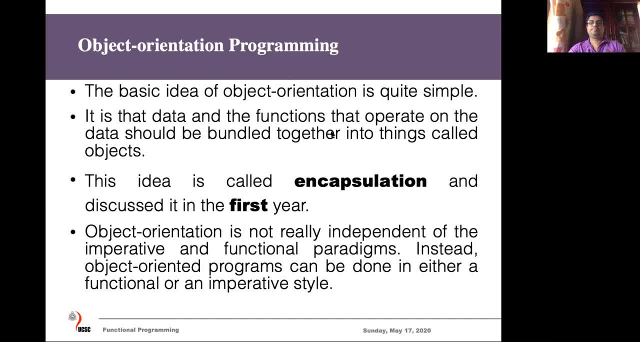 other method or other objects. so object-oriented programming is is not really independent of the imperative and functional paradigm is that the object-oriented programs can be done in either functional or imperative styles. so if you want to develop object-oriented programs, we can do it either in the imperative way or functional way. 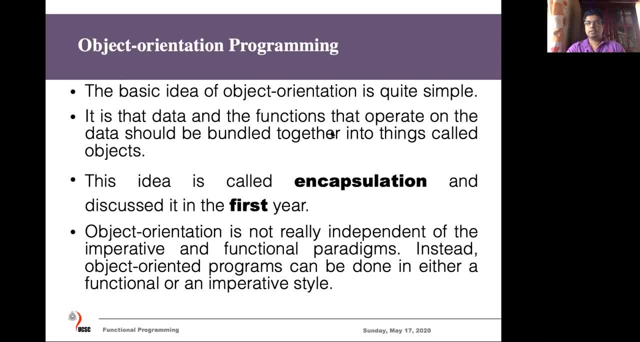 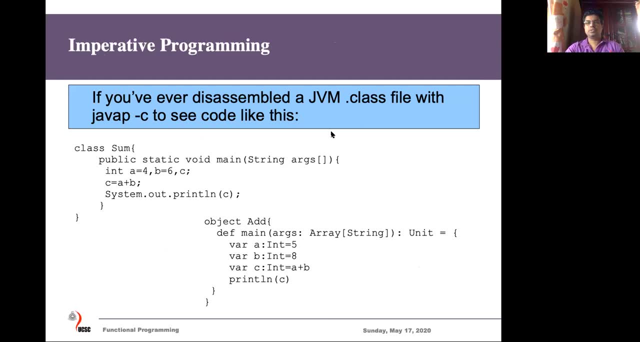 so objects are basically the method of encapsulation, functions or we call it as methods, together the data. so you know most of our Deadline should do something like this. so let's move on to the next slide. popular object-oriented programming in the world right now is java. so when you write a java program, 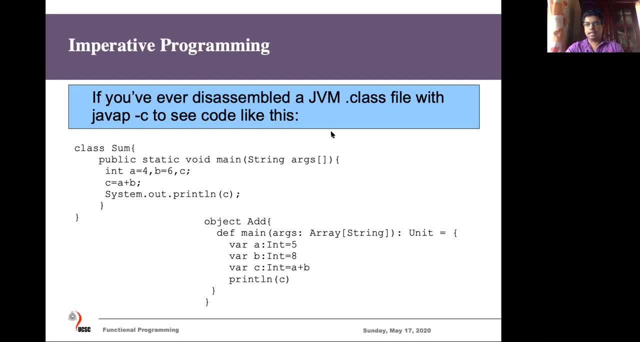 and compile it, create a class, java class- and you run that class in your application. so we write the code. maybe if you want to add something, we will write a code. maybe call some and it has the method main. this object is called, it has some and we define that object called using keyword class and inside that object there is the method. 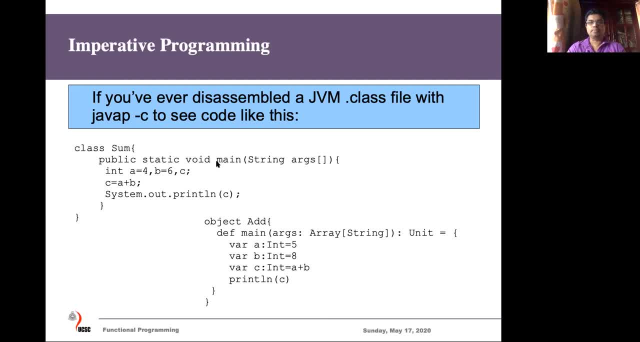 called main method user. anyways, of option. it has input called string input which we can give it and inside that we have some variables defined and, uh, some values are given here we add them and print them value on the screen. So, similarly, if you use some other language to do the same thing, 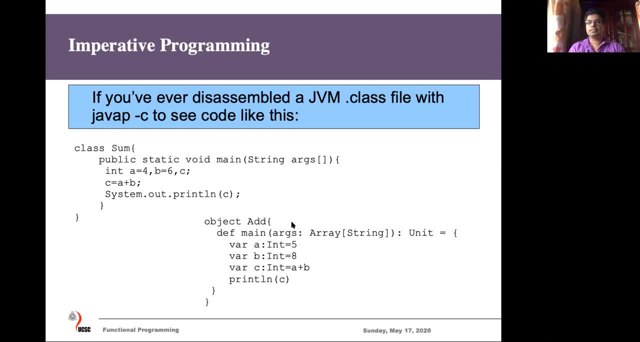 we can write that same function or same action in such way. So then we might use different compilers to compile that to the class. So maybe have you get a chance to see the final instruction says so in the file called java class file. So if you don't do so, maybe using a. 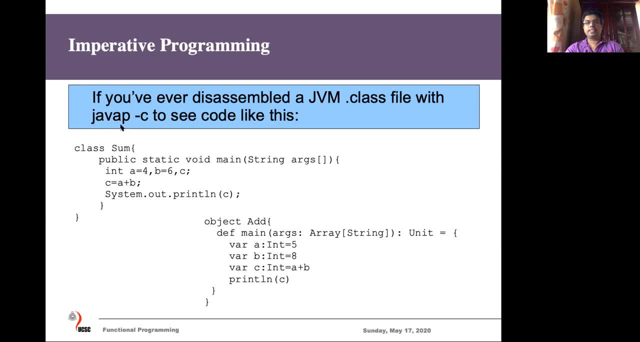 tool called java p. So you execute java p minus c and then you give the class name. it lists down the java vm instructions. So you know java is a virtual machine. so you, whatever the code you write in java, compiled or converted into the set of imperative instructions. 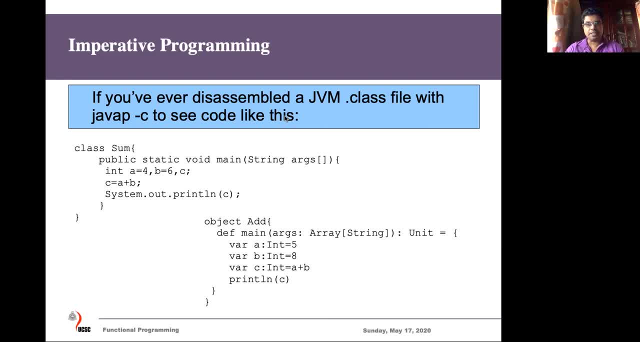 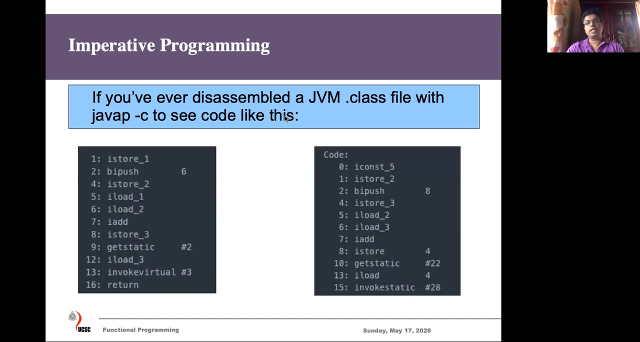 So those instructions defined by the java specifications. So then the java command, or what you call it as java interpreter, further interpret or further convert this java vm instruction into the java p to the corresponding machine instructions. So you can see java vm instructions if interest. 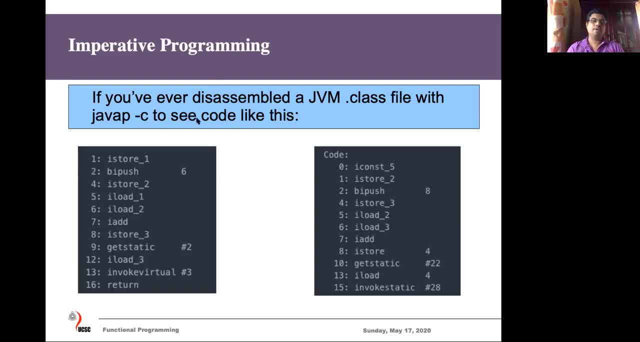 using this java p minus c command. There you might see, all these java vm instructions are imperative sequential instructions, one after other. So if you want to add, you might see, say, store some values and then load those values into the memory and then execute add instruction and then store results in the java p. 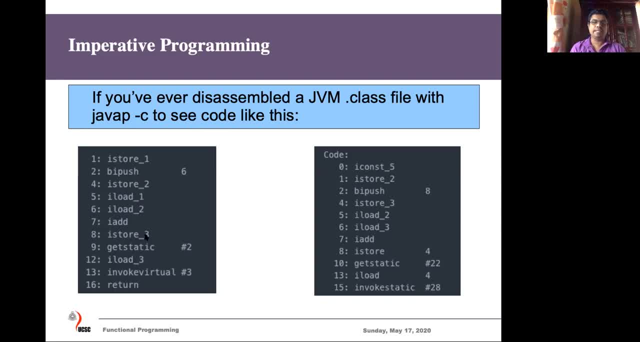 and then store results in some location- they name it as three- and then maybe load. using this, they say load print methods to print those values, Whatever language you used to pull. finally, it ended up with similar imperative instructions. Computer execute those one after other. So, as you may see what is, 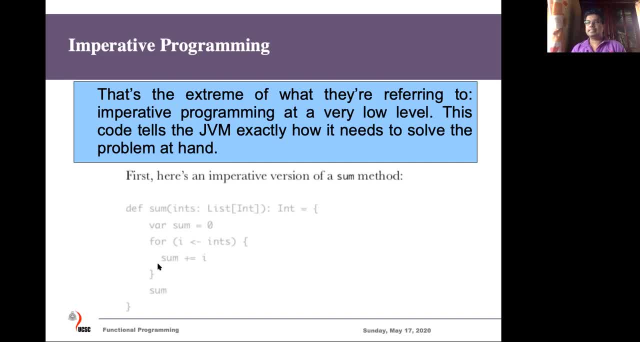 happening here is that functional programming is kind of writing style, but in the low level it's sequential execution in a computer. obviously do we do some parallelism in some architectures. So in order to further understand what I meant- this programming styles- let's have a look. we want to add. 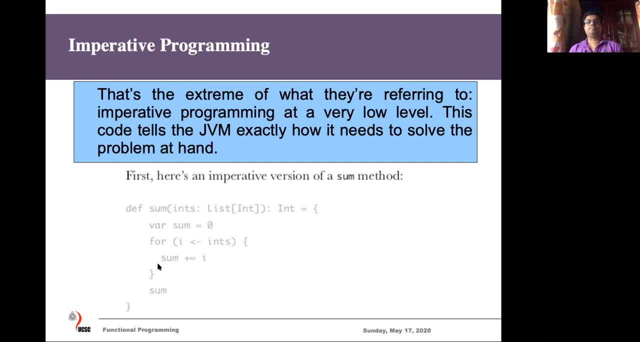 sequence of numbers store in the array or what you call list. So, in the imperative style, if you want to add sequence of numbers which is store in the list, then we need to instruct the computer. please take one number by number in the list and add them. 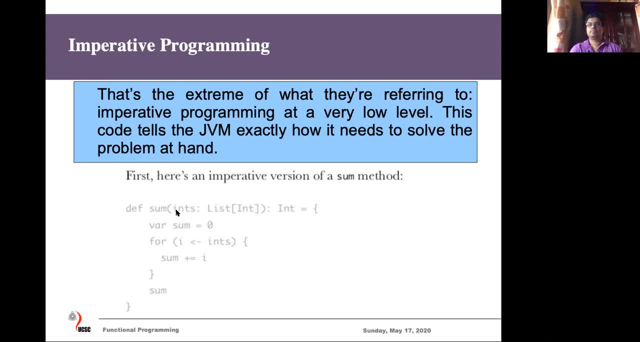 together. So basically, you know from the beginning what we did. We create a variable to store the total and we write a for loop and take the numbers in the list one by one and add that number to the list. or the variable for sum, add that number to the sum and store it in the sum and we then take the next. 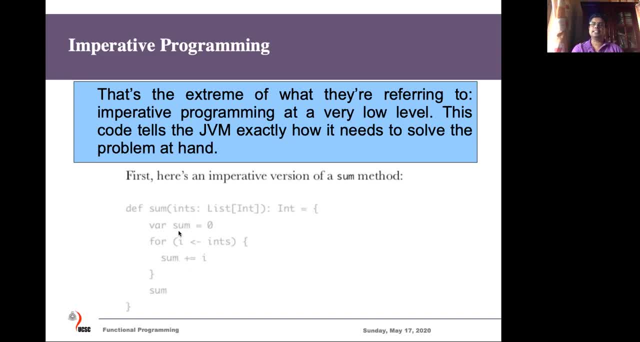 number, then add it and store. So take the next, add it and store. So we tell the computer how to edit. So we say our data is in array And we are going to take one number at a time and add that number to the results and store the results back in the 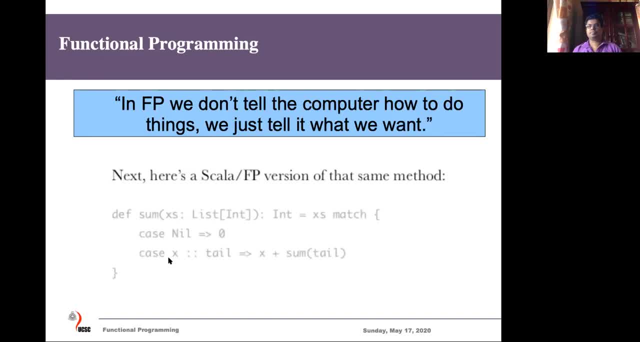 result space. So if you want to give the same set of instruction using functional programming, we are not telling the computer how to do that. tell the computer what we want. so what we want is the addition. so in the functional programming we can define our addition something like that we can say: if the array is empty, the sum should. 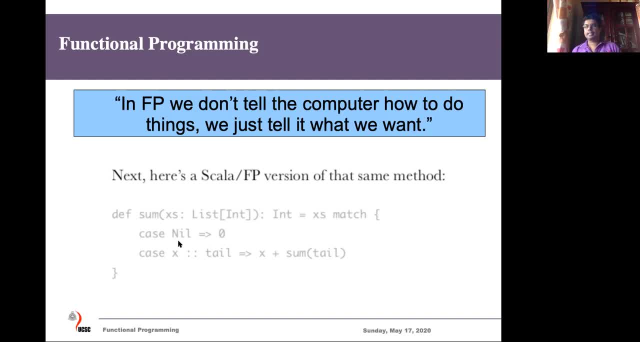 be zero if it is not empty. sum is adding the first element to the rest of the elements- recursive, obviously- so we can pass some instruction like that. so if you pass the instruction like that, so we call it as a functional state. so we will learn a new programming language called scala. 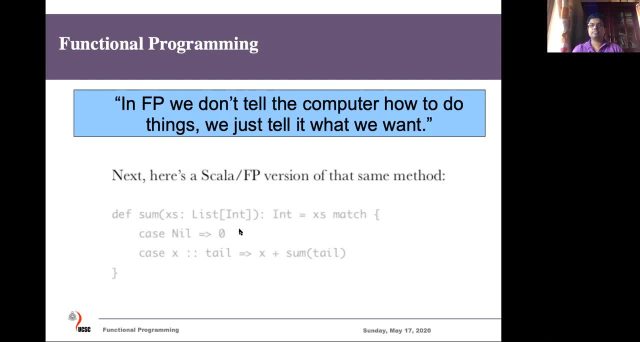 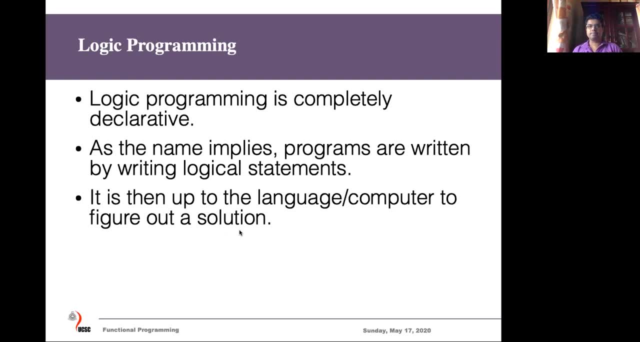 and we learn how to think like functional programming. so just to tell you about there is other programming paradigm for logic programming. so in the logic programming was so it has. it's completely declarative programming, like methodology. the logic programming also tells what we want. so most of the logic programming languages developed from the history right now. but 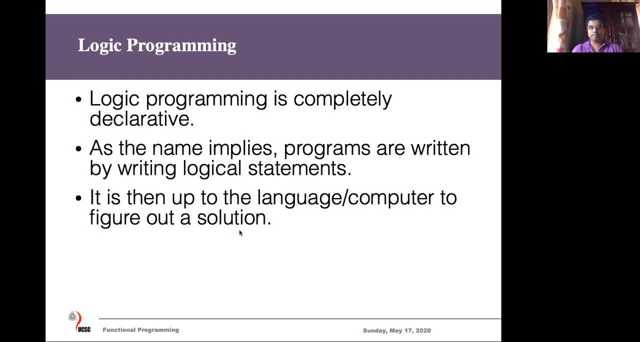 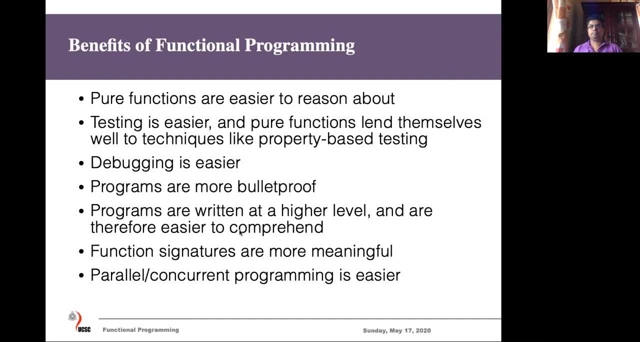 so those are not so popular about software developers. let's have a look. what are the benefits of function and program? so the main benefit is those functions are very small, easy to understand, easy to reason about and easy to debug and obviously test after test step and we understand. 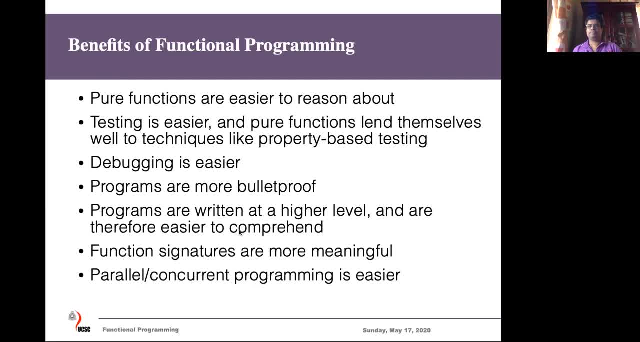 the input and output is correct, that's correct forever. we may not face any bug later on, so testing is perfect. but in the logic programming we learnt that to use functional programming orhei can's. so we, when develop the functional programming, we use the meaning to names for their functions, because of thelighting, because the functions have function here. 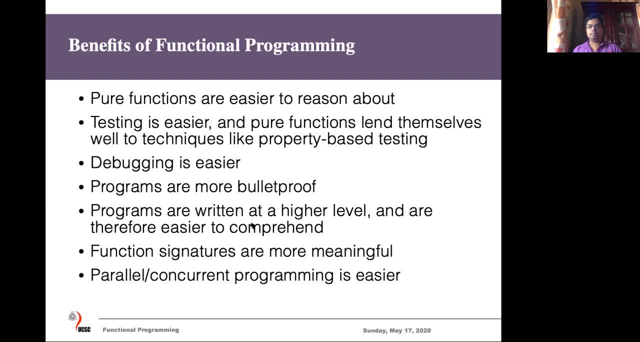 of that credibility of functional program is much more better than structure or the imperative program and when you want to develop parallel and concurrent programs, so it's easy to use functional styles. so if you ever develop such parallel or concurrent program you may understand why I say so. 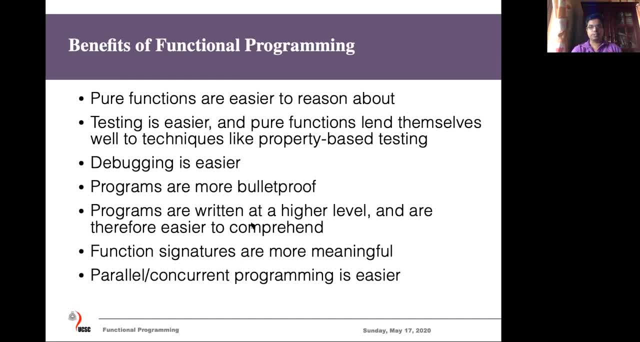 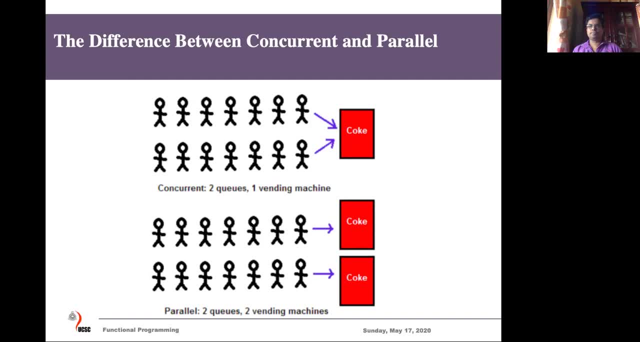 so obviously you will learn that in this course, so then you may understand what I means. so before that, at the introduction, so just to give you idea, parallel program and concurrent programming is two different things, different between parallel and concurrent- can understand by using this simple diagram. in concurrent programming it tells about sharing the common traces. 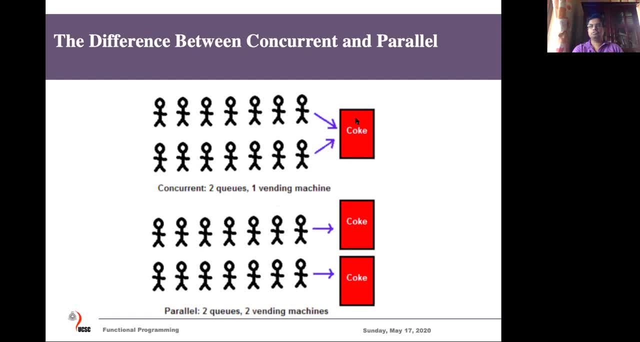 there are several parallel entities which want to access some child resource. so, for example, there are two cues of humans want to get coke from the machine, single cork machine. so then there should be a way of accessing the single core question in the favorable, fair way of accessing that machine. 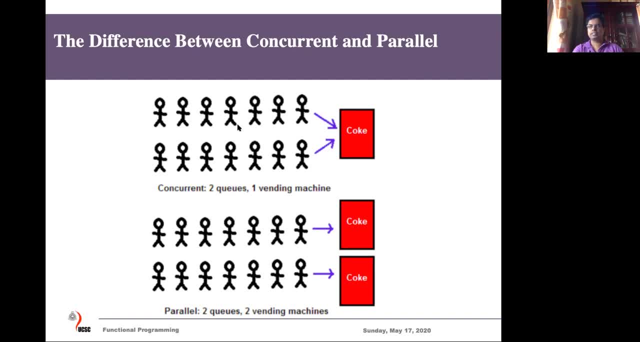 for the both cues. so those things we consider on the concurrent program, how to access your resource, so that is we call usually in control, so in the parallel programming. so those cues usually independent. so there are two code machines below two cubes so the people will take force. 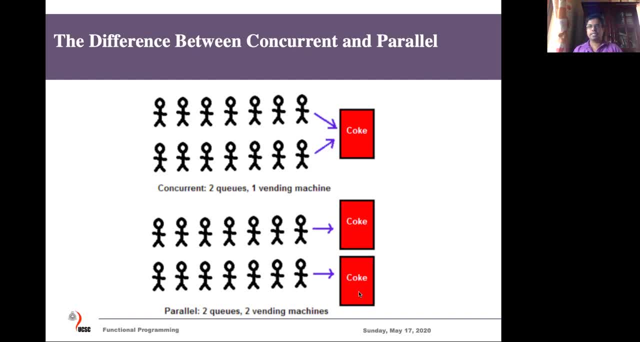 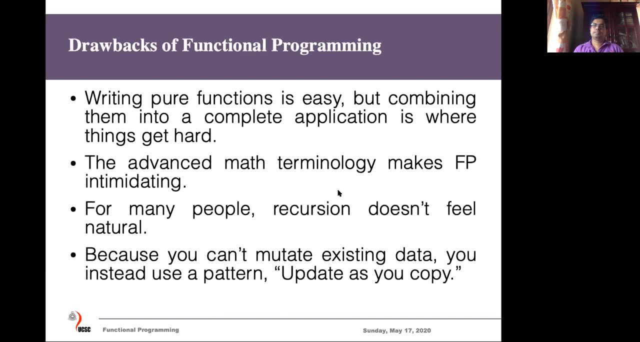 independently from two different cues so they take at the same time. this is parallel. this is confirmed. obviously, when you do functional programming there are drawbacks. the main drawback is: writing a pure function is easy. if you want to combine those pure functions together to build a big applications, maybe it's confusing and hard and people have issues. 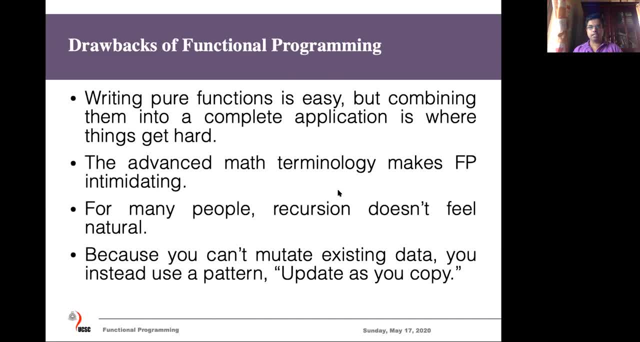 on understanding some of the terminologies that are used in functional programming, especially like concepts such as recursions. that doesn't feel the humans, because in the human world there are no recursions. happens kind of in their brains. so in the functional programming you show you updates on your copy. so there are no global 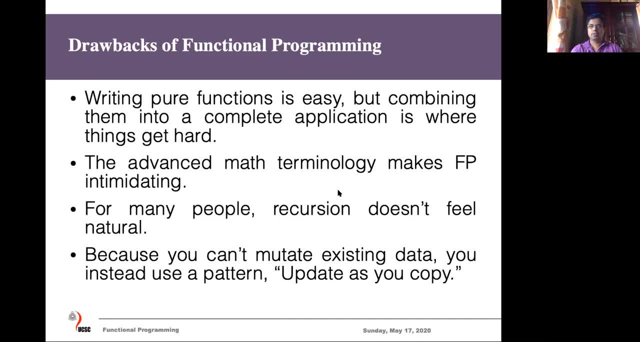 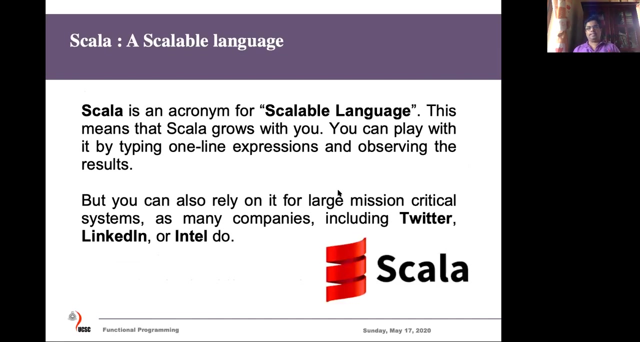 states or update states and so on. so typical programmers are feel uncomfortable of those styles sometimes. but if you do implement somehow real functional program so they are much efficient and kind of error proof. the main thing is error proof because those programs builds using small, small activities. right, i think that's enough for the internet introduction. 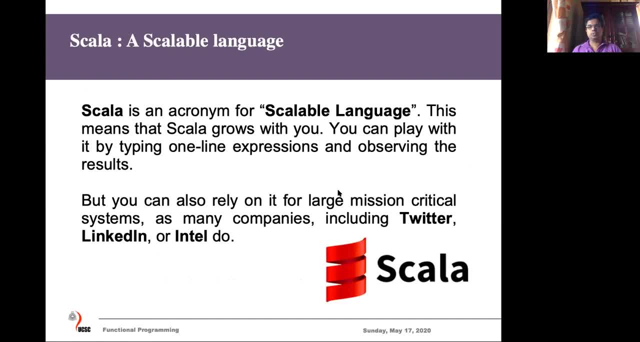 let's introduce the tool i use to teach functional programming. so in history, right now in the computer science world, there are several functional programs that are used in functional programming languages. so among those programming languages, i decided to select scala as functional programming language. scala refers to scalable language. using the scala, we can implement. 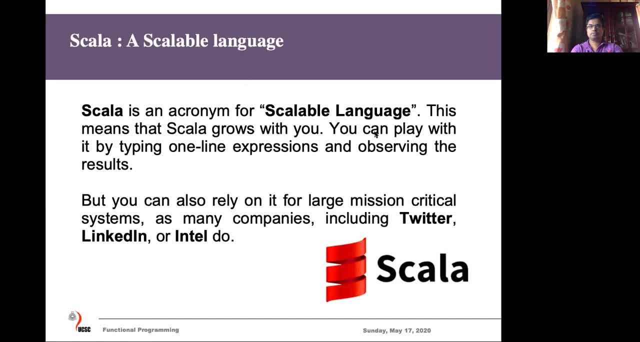 programs in the object-oriented styles as well, if you wish so. finally, those scala programs compile to the object-oriented programming language, so i can use the object-oriented styles as well. if you want to introduce a program in one robot, you can use your own private hardware plate or your own. 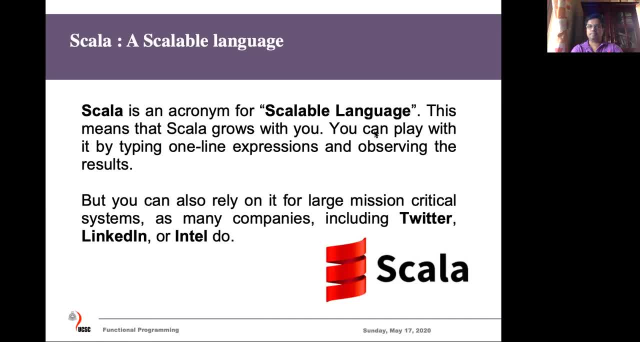 kinds of Günther machines, as well as any operating system where you have point 1 meansă, which are simply two already used tools in the very early days of scale. we're not gonna for the basics because, by the way, about scala it's the own, control software it's own. 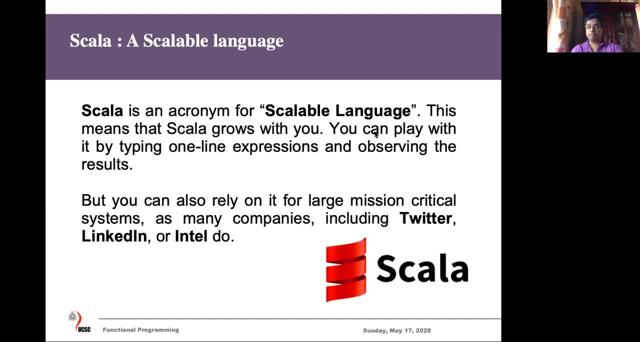 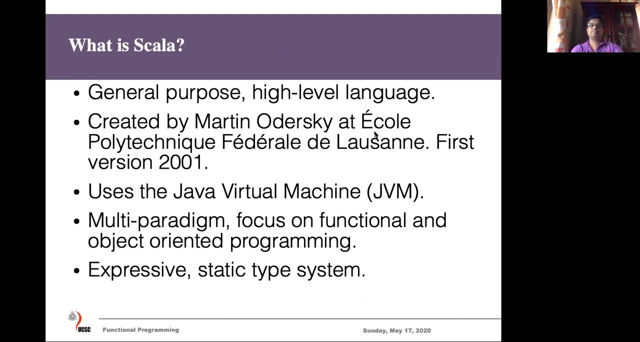 To develop backends, especially when you develop conference and parallel programs Distributed way, Scala is the best language to use. So Scala has a general purpose programming, high level programming language created by Martin Ordesky somewhere around 2020 years ago, So the best part of it: this language compiles the code to the JVM. 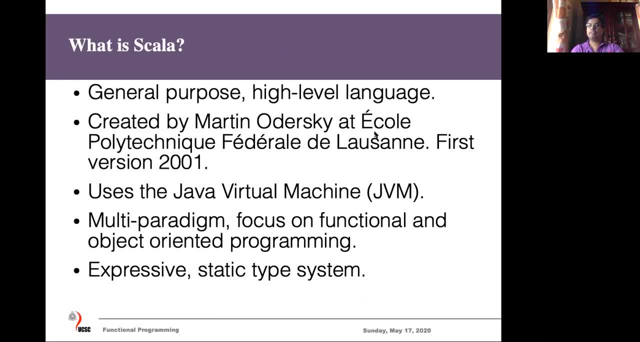 So you know there are a couple of programming languages which compile. finally, on top to the JVM, Kotlin is some other, I guess. So Java is obviously the first language which runs on JVM, But people have developed different programming languages can also use to write programs. 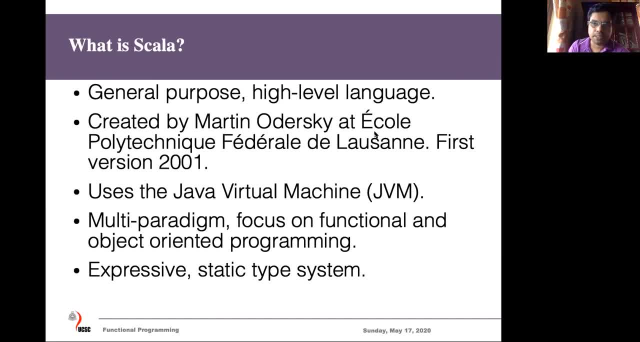 And finally, because Java's specification is open. open specification: anyone can develop a new programming language which compiles their code to the JVM. So in the Scala, what they did? they combined functional, object-oriented and all other programming style into the one set of programs. 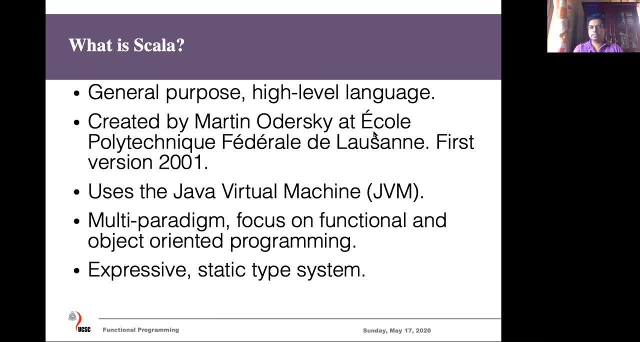 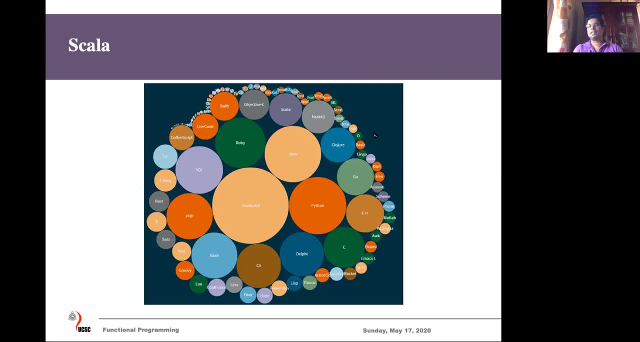 So we use Scala to teach only functional styles In order to understand the positions of Scala. so I just show you this diagram Right now. some people say most popular programming language in the world is JavaScript. Some people say it's Python. So, by the way, Java and JavaScript is two different programming languages. 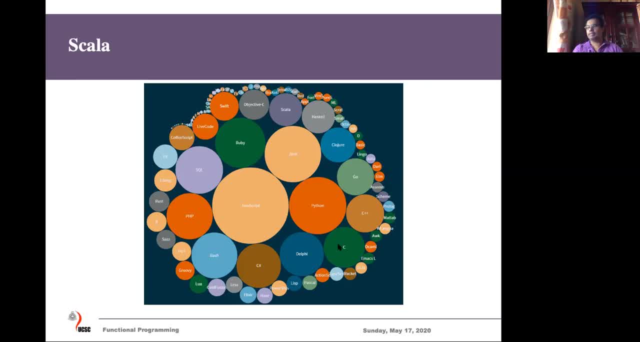 JavaScript's mainly used on the web developers And Java is used for backends plus web plus whatever other applications. So nowadays, as you may notice, Python is getting very popular because of its simple styles and huge set of libraries available. But obviously there are no doubt Python, Java, JavaScript are the three most popular programming languages in the world. 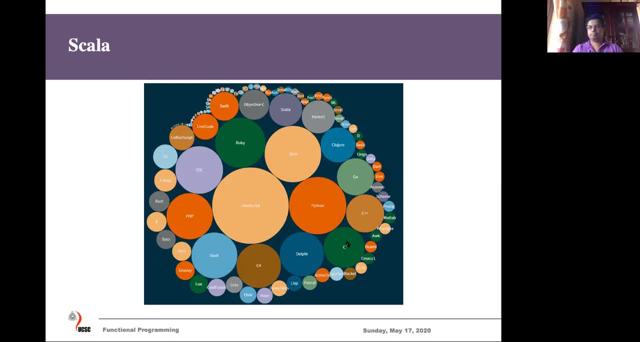 But we cannot forget about C. C started somewhere around the initiation of computer science, but still survived. So obviously developing a C program takes time, but the most efficient programs in the world If you want to have game engines, operating systems all developed using C. 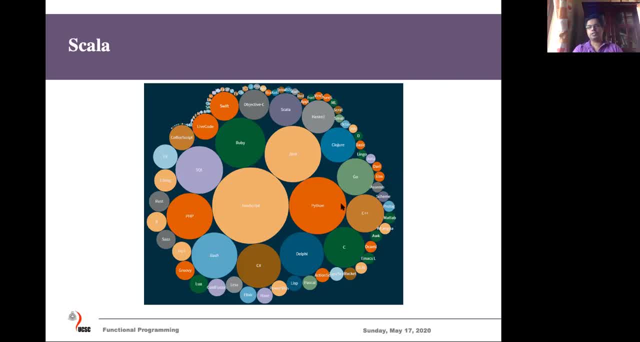 So we have to pick our programming language based on our type of application. So in this cycle, when you think about Scala, Scala may not get a good percentage out of this cycle. So you see somewhere here. So there are similar popular languages available right now. 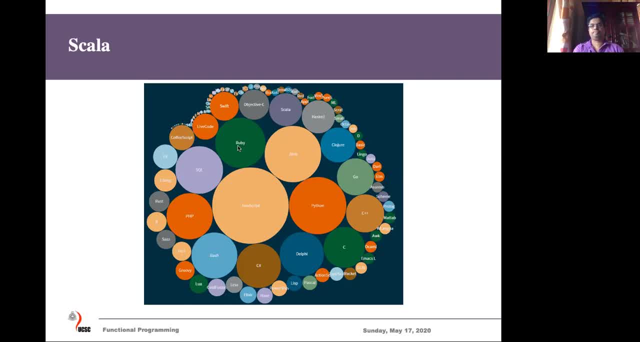 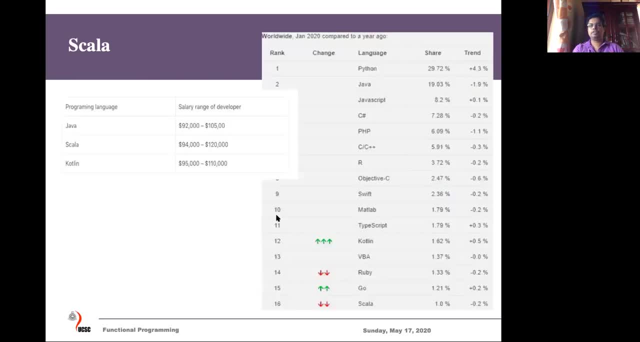 One is Go and so on, But people think it might get popular. So in previous back it was kind of getting popular. But when I checked in 2020, it kind of popularity- The rate of Scala kind of going down, similar to Ruby on Rails as well. 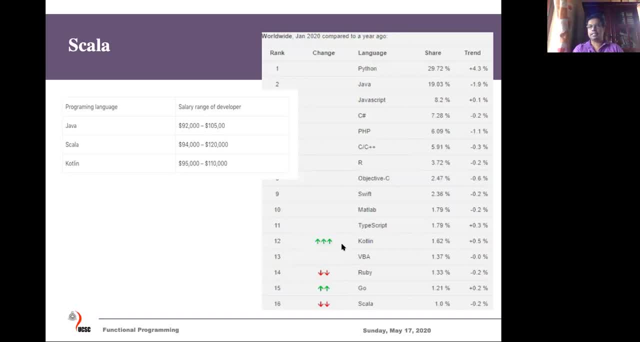 Like languages like Go and Kotlin is getting popular, But I still decide to use Scala to teach you functional programming. So obviously, Python, Java, JavaScript, C, Sharp- They are the most popular language in the world. In 2020, Python was the leading language. 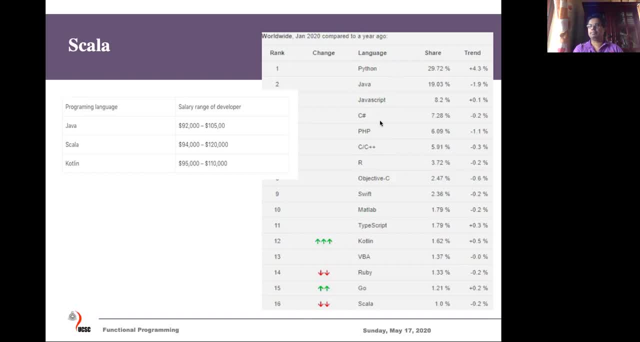 And Java. JavaScript has similar portions But when you take us, Scala-like language has a very small portion of the popularity scale But due to their features and due to the kind of like their features very important in developing concurrent and parallel applications. So the learning functional program such as Scala is very important in this century or in this era. So in order to prove that, I kind of put you the salary scales of a software developer in US. So usually Java developers get $92,000 to $105,000 per year in US. Scala programmers get up to $120,000 per year is $10,000 per month. Finally, the highest salary Because there is a demand in the mission-critical application development areas And parallel concurrent application development areas for the functional program or functional development. 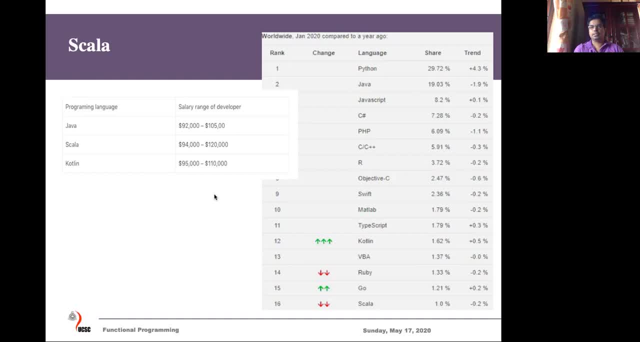 Software developers who know functional programming, But the demand is high even though this portion is small. There is a high demand for such developers, But there are very few people who are on that, Especially with the data science applications. So functional program has very high demand. 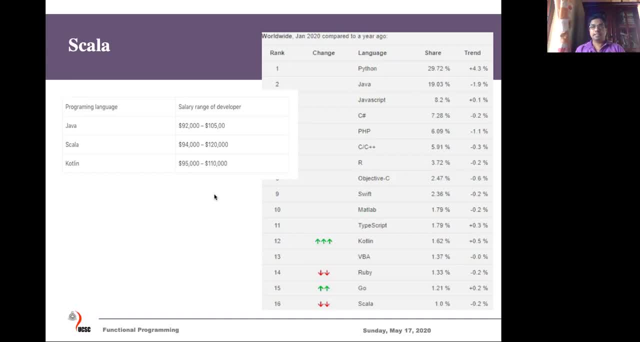 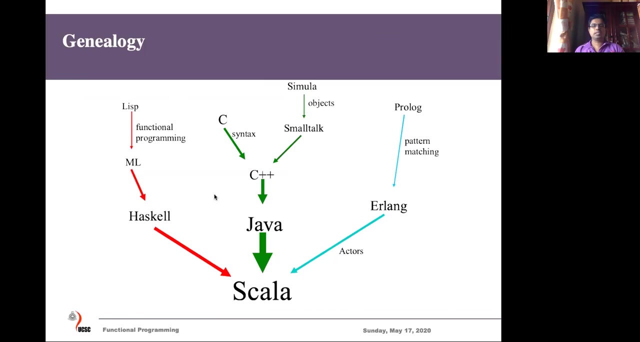 So we will learn how to do those things when you move on. So you may have heard about Apache Spark in the data science area. So they use Scala. So Scala takes the good properties of all the programming languages in the world into one programming language. 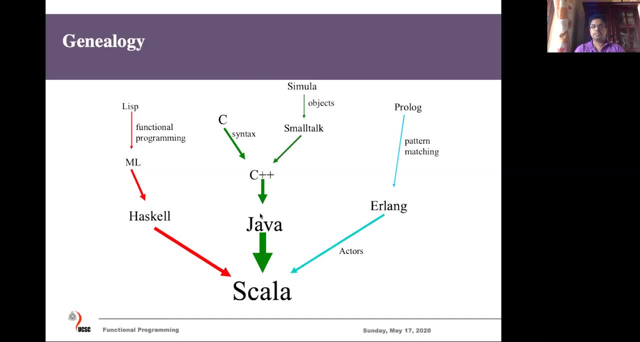 They inherit some features from Java, Object-oriented features. They inherit some functional programming features from a functional programming language- First functional programming language in the world- called Lips, ML, Pascal, To the Scala And they have taken some good pattern matching features from all of Erlen's and to the Scala. 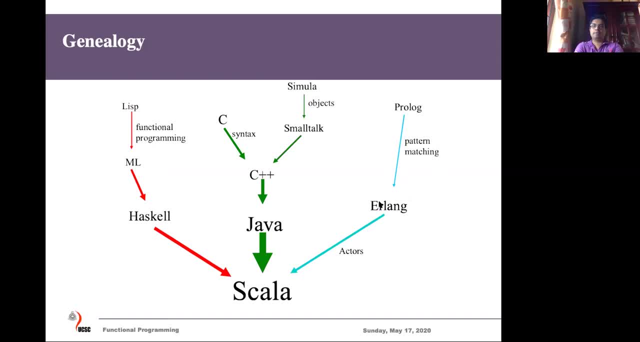 So there is another stylus of doing developing parallel programs called Actors. So you may have heard about threads So similar to that. there are methods of doing concurrent and parallel programming called Actors, Which is used by a language called Erlen. This language is heavily used by telecooperators to develop SMS switches. 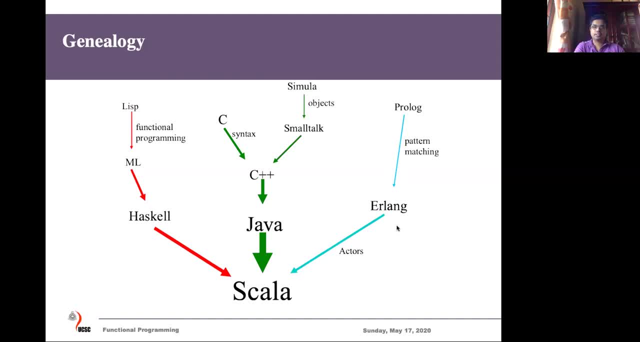 Like for mission-critical real-time applications. So, using Scala, we can use Actors, We can use Objects, We can use Conferences. So that's why this language seems to be really powerful. So when you develop a program in functional style and Actors-based using Scala, 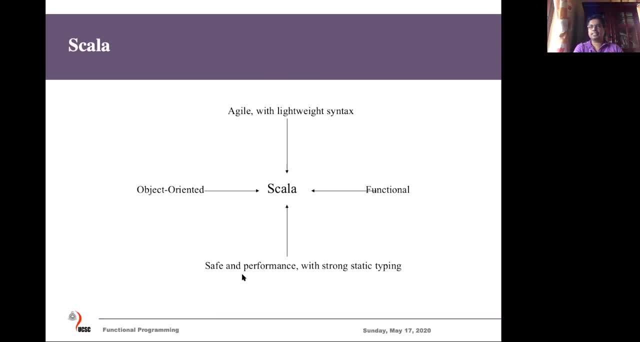 So it is very, very less charged. It has some bugs, So it's kind of inherently secure And their performance is inherently optimized And so we can write such Scala code In few lines. So where we need to write Java code in 100 lines, 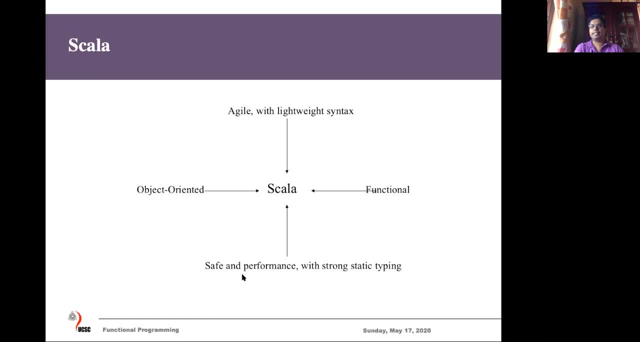 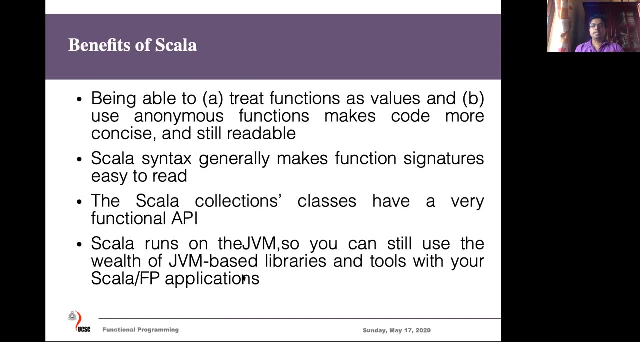 In other words, 100 line Java codes can be written in Scala in 2-3 lines. So obviously that's good to learn, right? So I use Scala, as I said, to teach you functional programming. Because of that I am not teaching you. 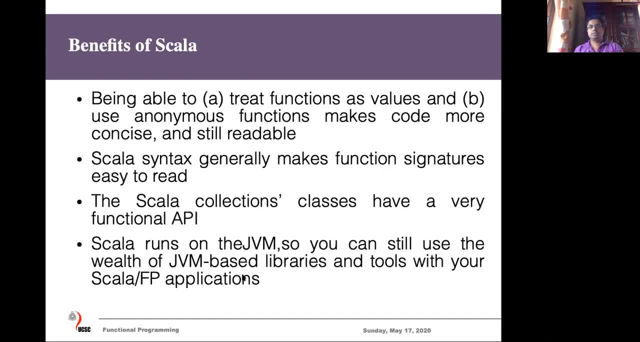 Scala, So you yourself should try that To learn this programming language. So benefits I highlighted, Since it's functional style, we write error-free codes. And the other main benefit is Scala programs run on top of a Java VM, So existing old Java libraries we cannot use in our Scala. 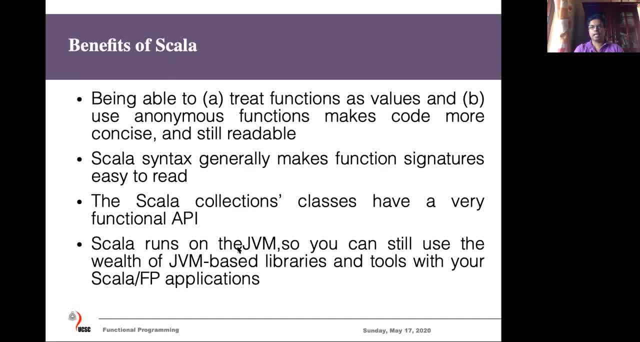 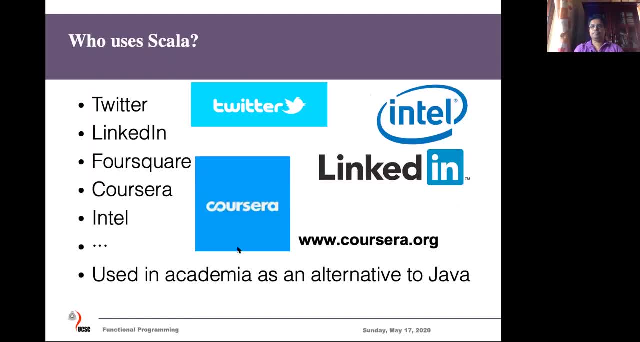 And Scala codes runs anywhere which has Java VM I mentioned. who uses Scala right now with their backend developments like Twitter, Implemented by Scala. They are the main people who are behind the Scala, Their entire backend developed by Scala And Coursera. like organization linking is intent. 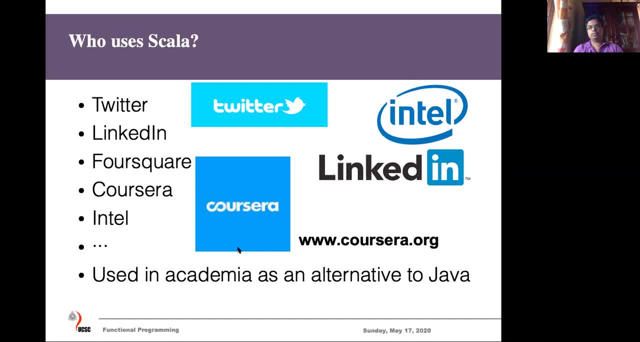 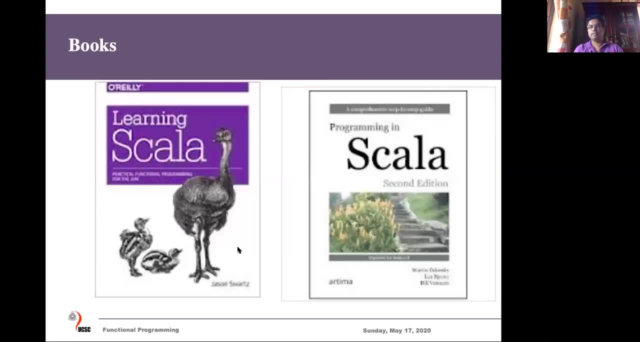 They are heavily used: Scala for backend, Backend developers. There are books available in electronic form as well as printed form. Two of those books I highlighted here, But I have uploaded one book to the LMS, So that's enough, if you can read, to learn functional programming style. 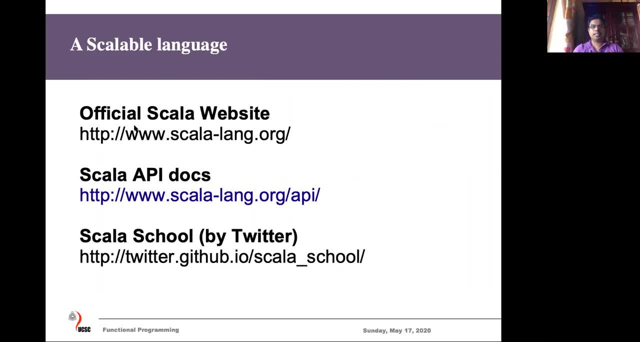 Here are the official websites, Scala language warranty And the API documentation. you can go through this URL And the Twitter are the people who are mainly funding this Scala development or the Scala warranty, So Twitter has a separate page for Scala school to learn Scala. 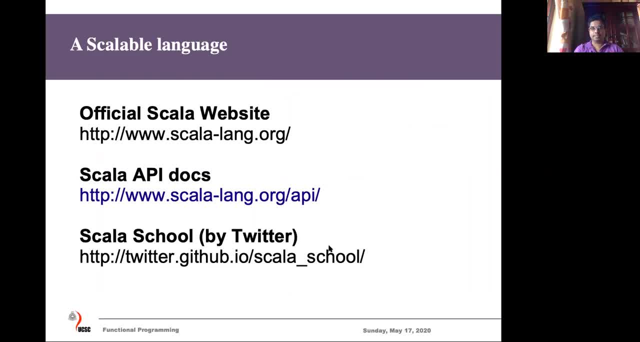 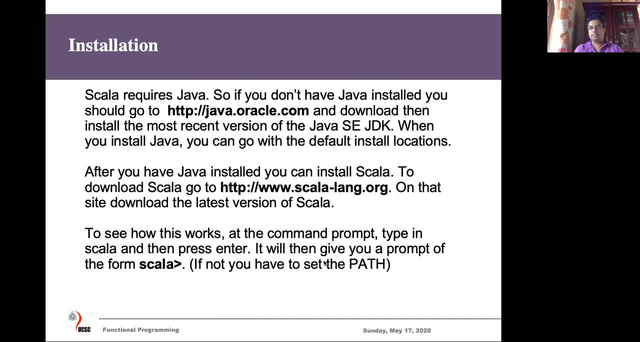 So these are the resources where I should start this journey. So you have to visit those things to go through this journey. In order to go through this journey, Obviously, when you want to use Scala, you have to install the Scala. Scala runs on top of the general Java VM. 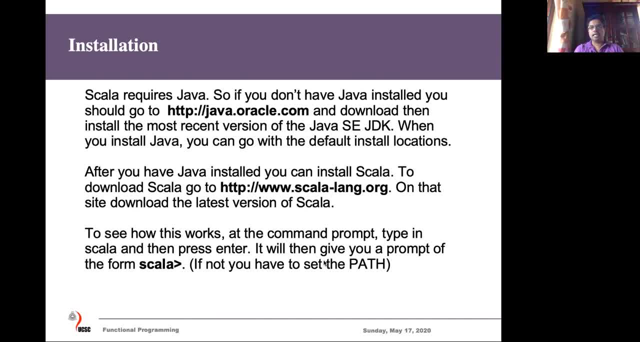 So you have to install Java, I think in the present Scala. I want Java version 1.8 or higher version SDK installed in your machine in order to use Scala. So, in other words, there is a built-in tool of Scala called SBT. 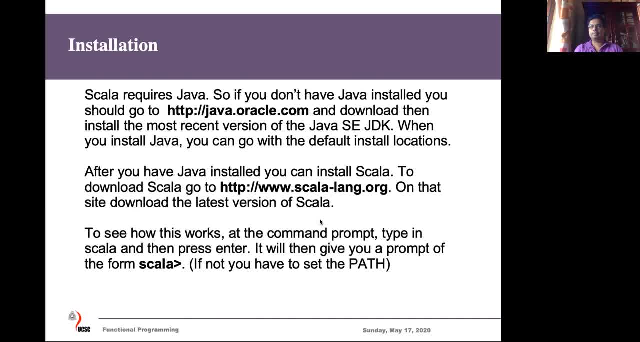 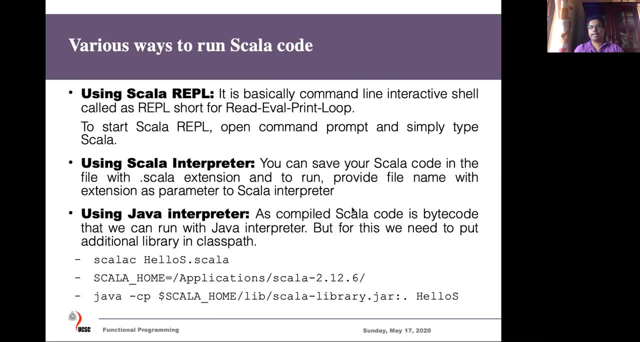 Simple build tool. Now they call it as Scala build tool, SBT. So by installing SBT you can automatically install all those things as well. So there are various ways to run the Scala program. So most of the time I am using REPL. 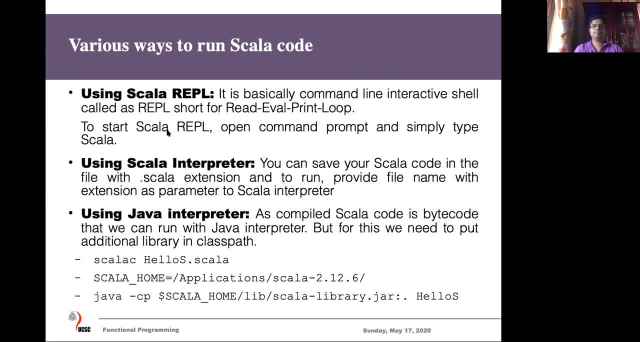 For what you call it as shell: Read- evaluate print loop For the shell of the programming language For: read- evaluate print loop For REPL: REPL prompt To show you the styles. But you can write, develop or write a code as a text file. 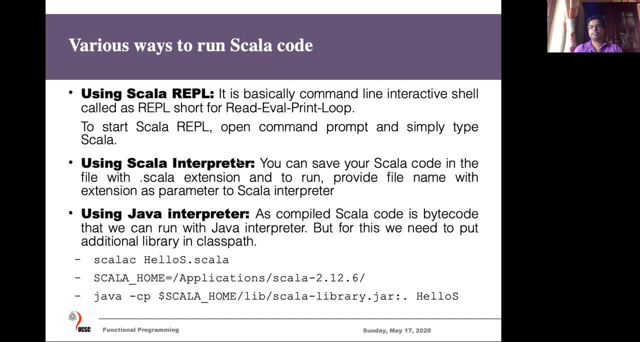 And save it, Compile it and run it as well, Using Scala command Like similar to Java, Similar to Java commands. So, since it's on top of the Java VM, After compiling Scala code, even you can use a Java to run that. 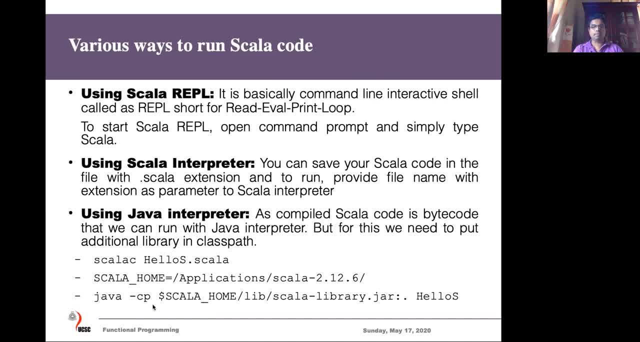 So if you want to run the Scala program using Java, You have to just give the Scala library And Scala code. This is, let's say, Scala code, Which can execute it by Java Directly. In the opposite as well, If you have a Java. 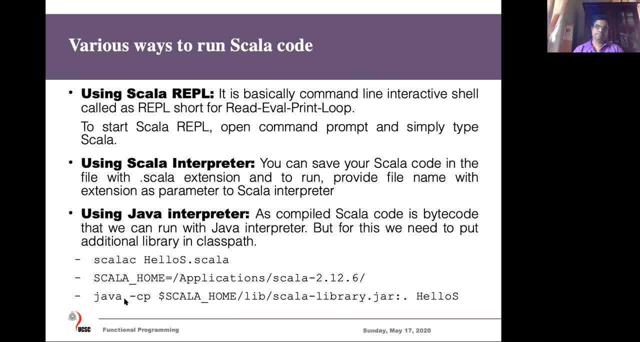 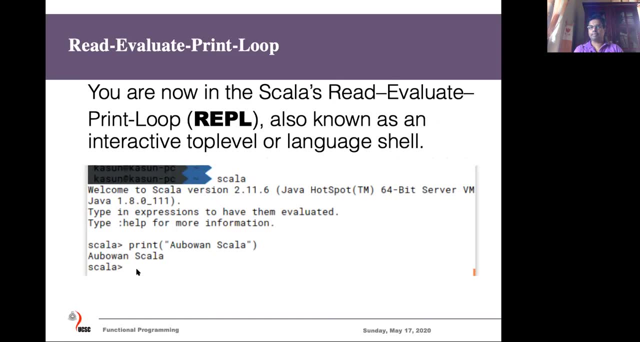 Using Scala command, you can execute Java code as well. Using Java command, you can execute Scala code Both way. These compatible each other. Read: evaluate print loop. It's a very nice way to learn programming languages. I use Scala Print loop. 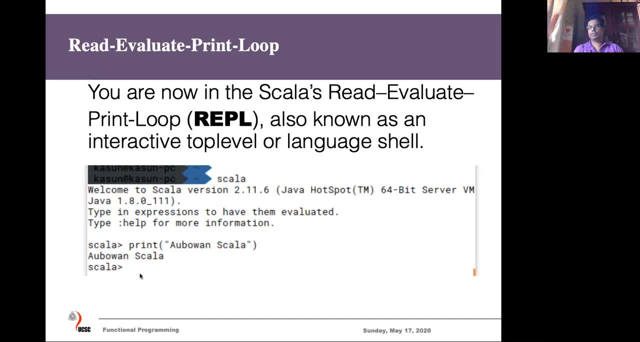 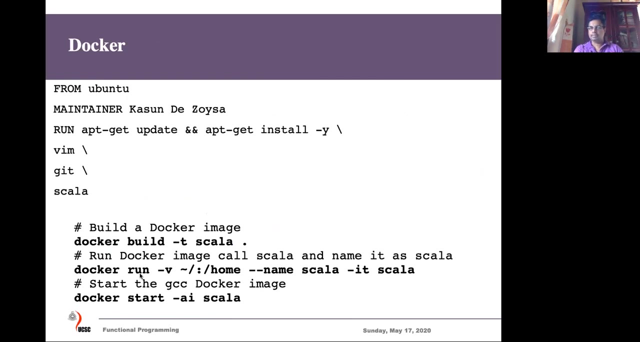 RAPL prompt To teach functional styles In the first few lectures. After that I move on to the serious real applications Where we can use some IDE. So if you want to restore Scala, There are several ways of installing Scala. 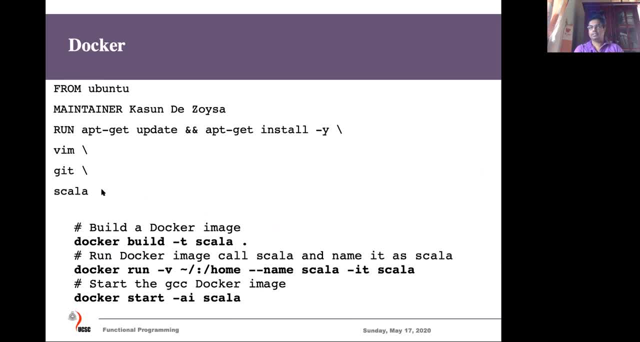 So simplicity, I have given you a docker file. So I think you are familiar with docker. If not, you should. So the docker is the new way of kind of Deploying applications. Instead of VMs, We can create what we call docker images. 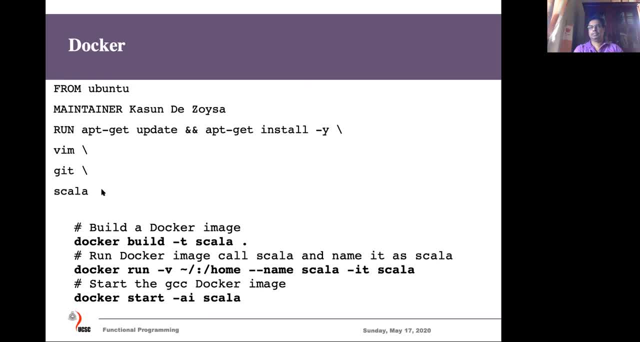 That is kind of lightweight virtual machines, So those machines Has what we require. So in order to learn Scala, We need small VM Which can run the Scala Compiler and interpreter. So I can build a docker image for that Using a base Ubuntu VM. 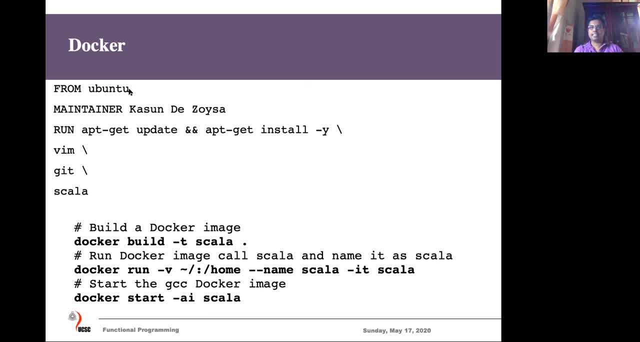 Which is in the docker file from Ubuntu. That means let's take a kernel of Ubuntu, Just a kernel without anything, And this is just my name, And then after that, Using docker run command And I tell Which kind of software. 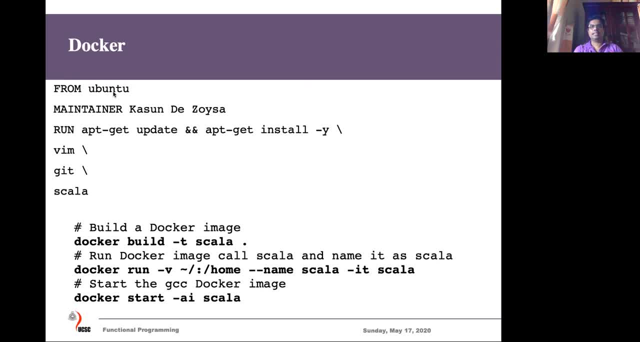 I want to install on this kernel Or this lightweight Ubuntu. So I say: update this Apg, update all the repositories. If you know Ubuntu, You know about apg update command. And then I say: After update, Apg, get installed. 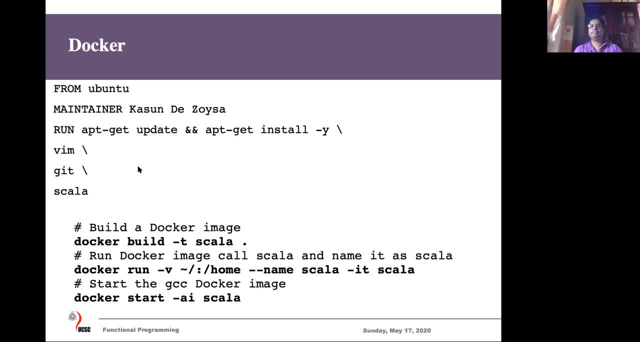 These three Things on that image For initial run, Initially what we need: A simple editor. I use Vim or Vi editor And I want to use You- I want to See you as in JIT- To manage your repositories. 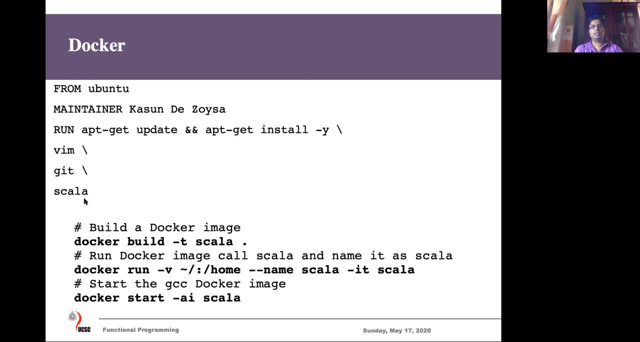 So for that I install JIT in that VM And I install this Scala. So if you run that In your machine, So you can Instantly build Ubuntu lightweight VM. What will docker image, What we call it as docker image? 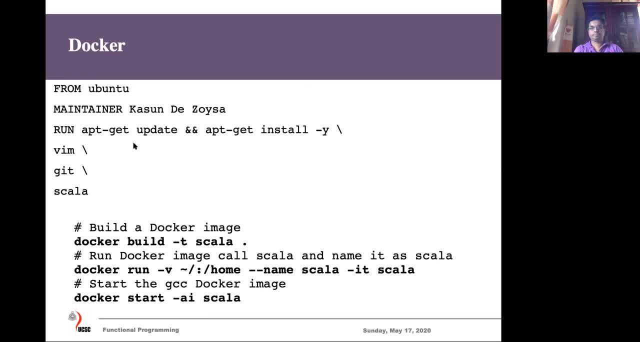 Which has the Scala installed on it In it. So if you want to use that docker, I will demonstrate in a separate video. So you put that file Into a directory And in that directory You run a command Called docker build. 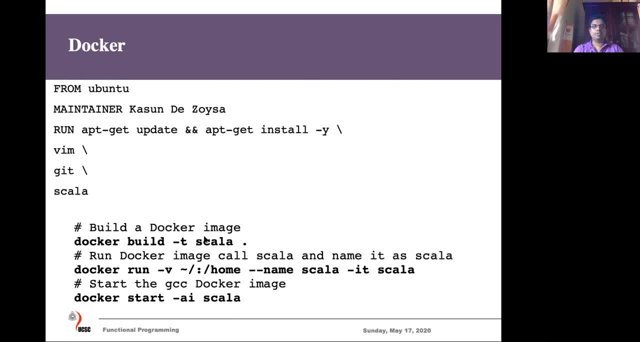 Minus t And give a name for your image And say root. So then the docker will see Check the docker file installed in the root directory And build A lightweight image Called Scala for you. This image consists of Vim editor. 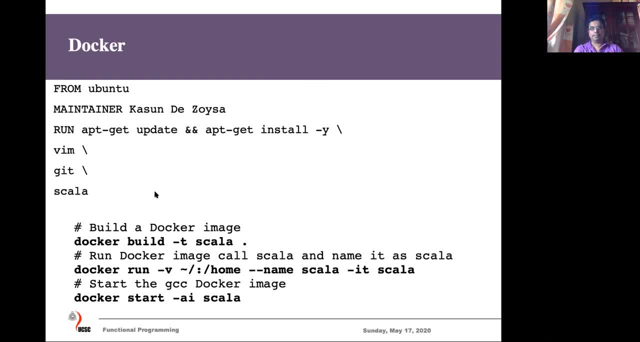 JIT and Scala Interpreter and compiler. Obviously, in order to run Scala, We need Java Open JDK as well, So after that We can run that image Using docker, run command Minus v parameter And we can add A host file. 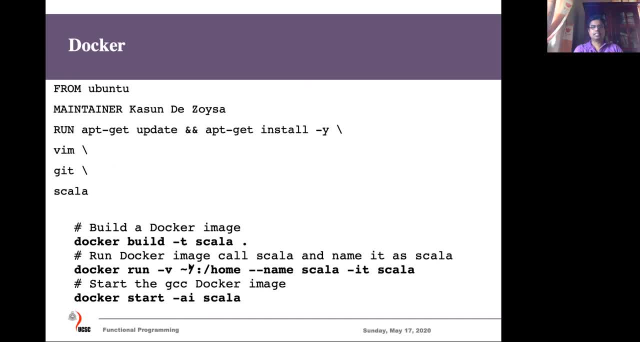 To the docker file. So I say Tildi, slash It has, take the parent directory Of my host machine And map it to the Home directory in the Vim. So when I start that Then Vim And change to the home of the Vim. 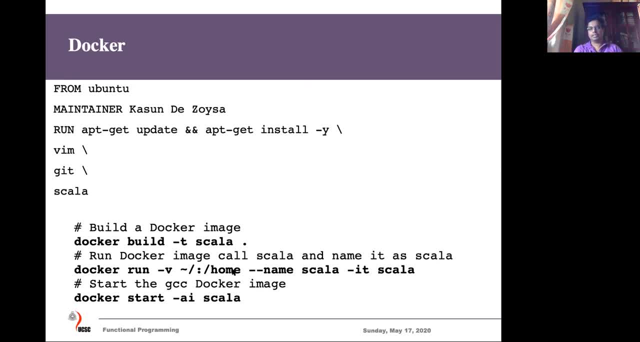 What I see is My Home directory of local machine And what I do with the image, Same did in my local machine. If you do it with Vim, We can't do that Because Vim may not see the host machine file system. 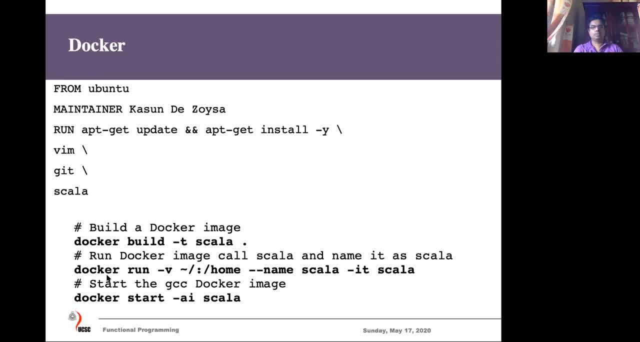 So when you use docker- Docker see the host machine file system. So how this syntax of the docker run. It has this mapping. If you don't want to map You can skip that, But it's better to map it And then using name. 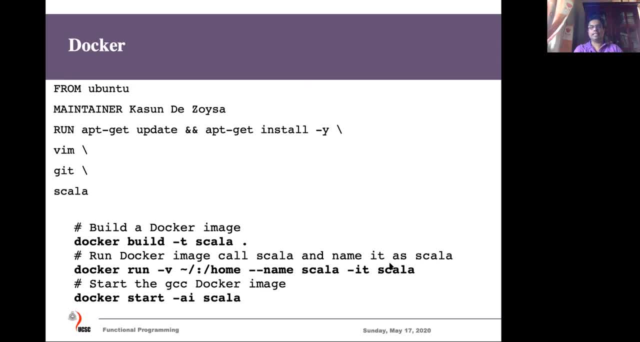 My dash, dash name To run And I give the image. So then it will create a Running image After you execute that. These two commands You want to execute only once. So after that, if you want to Start programming at all, 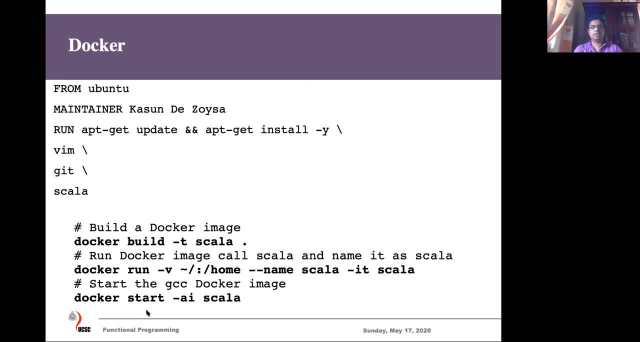 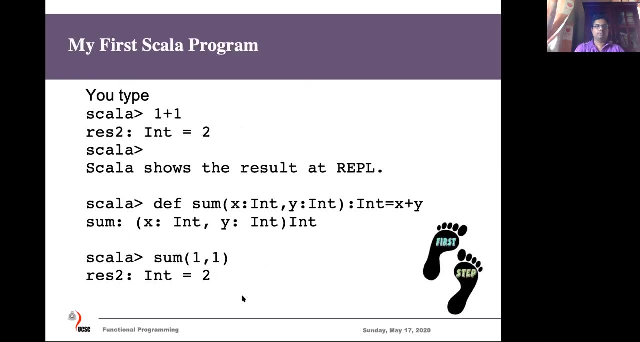 What you have to do Is start that image Using a command called docker start, And this AI option tells, After start that image Execution, To give me the shell. So then I automatically get The shell where I do programming. So this: 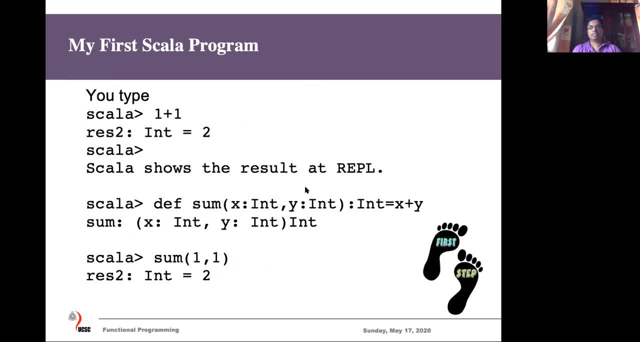 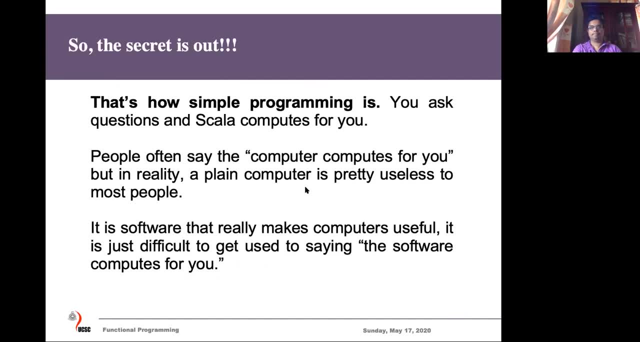 Tells you Simple first program. So I will create A separate video on this Demonstration, So I skip that. So that's it. So You, You simply now know what is programming is And what is functional programming is. 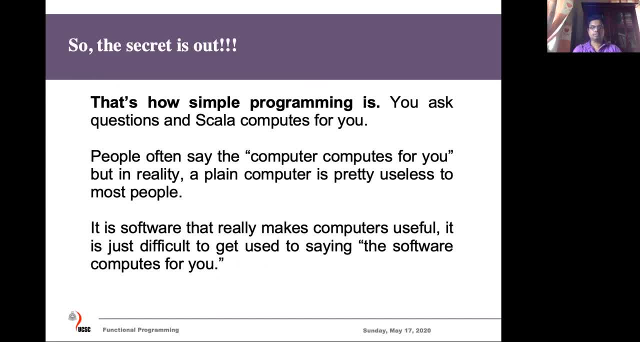 And what are the tool We're going to use those functional programming? Or to use What is the tool which we're going to learn Using learning functional programming? Scala is the tool, And so on. So, if you don't like, 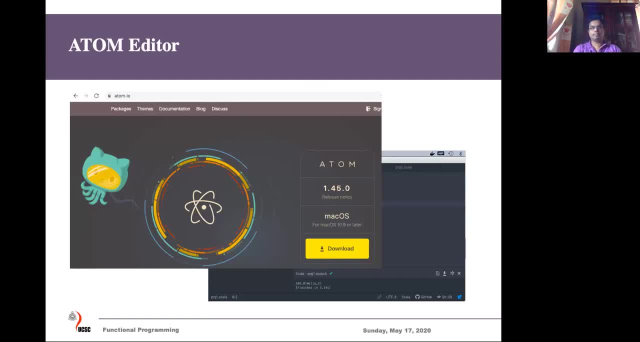 Formed VI and so on. So you have to use some Integrated environment IDV. So Atom Is the very primitive IDE Where we can use that to Develop any kind of programming language. It has plugins To most of the programming language in the world. 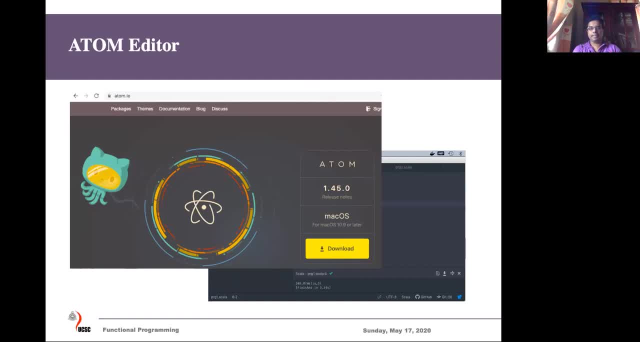 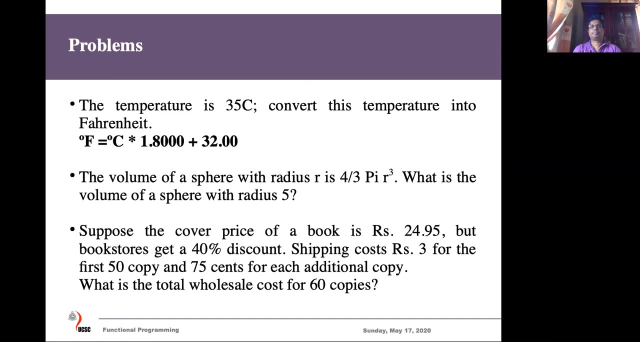 And simple editor. A simple editor. If not, you can use Heavy editors Like Intel J studio, Whatever editor- for Serious applications. So then you're supposed to solve These three simple programs As a start. So in the first program, 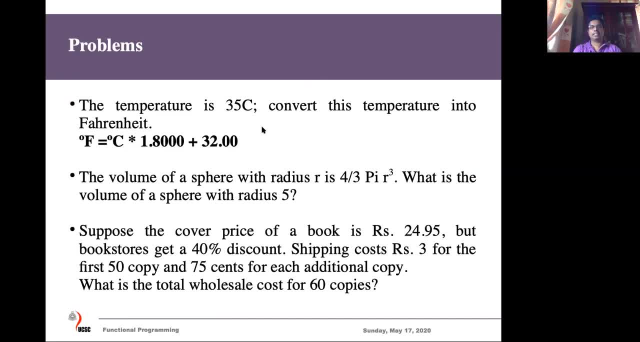 As you want to Implement a function Where you convert Centigrade into the Fahrenheit And in the second program, Say, you want to write a function For volume Of the space, Where I take radius as the input. It should produce the volume. 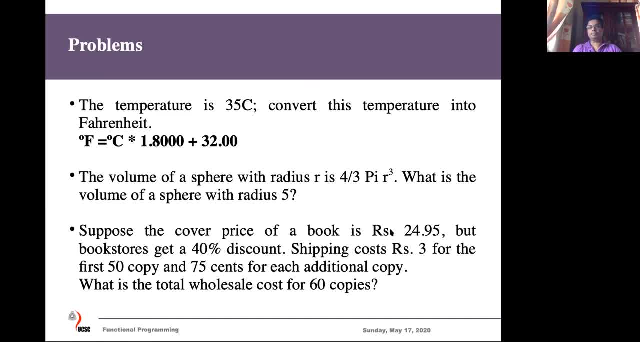 As the output And then in the third It gives some problem And asks you to implement. So these three things Are your homework. I will upload this as a Assignment, First assignment of this course, And you can follow my. 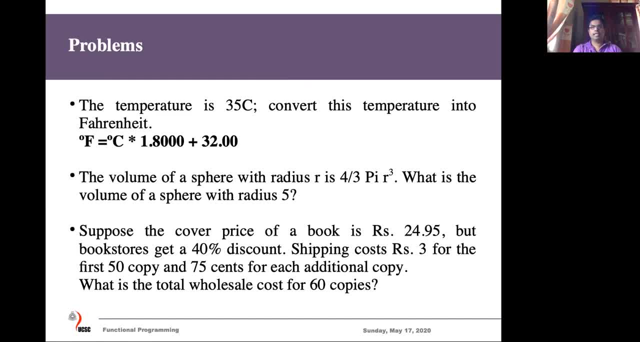 Second video. It's a demonstration, And do code this And upload It to the LMS. I will Show you how to solve Few problems in the second video, Not all When you are uploading Assignments in this course. 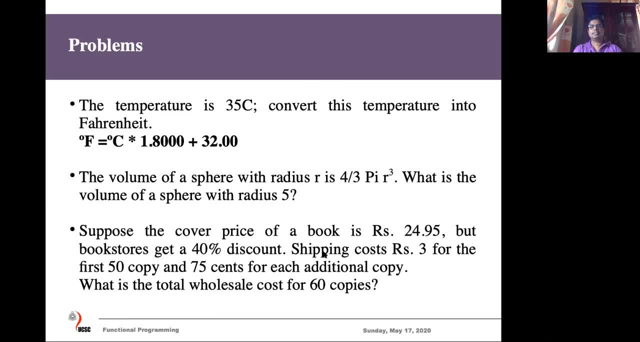 I am not accepting Direct submission of the course. You have to create Your own JIT account. Either you have to use Jithub or Jitlab. There are two online repositories Nowadays get popular. One is Jithub, Other one is Jitlab. 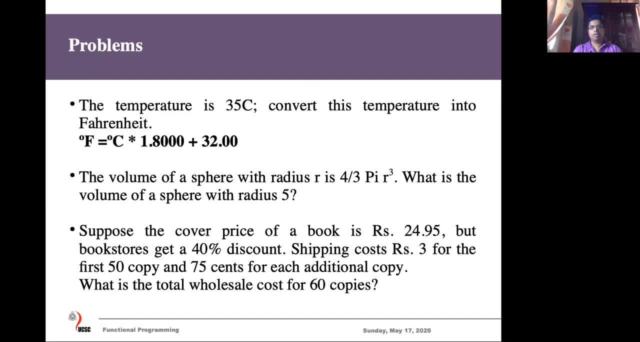 So I guess You already have Assignments in one of these. If not, Create an account with Jitlab or Jithub And create a repository For this particular course. New repository: You can use any name. Maybe you can use functional programming. 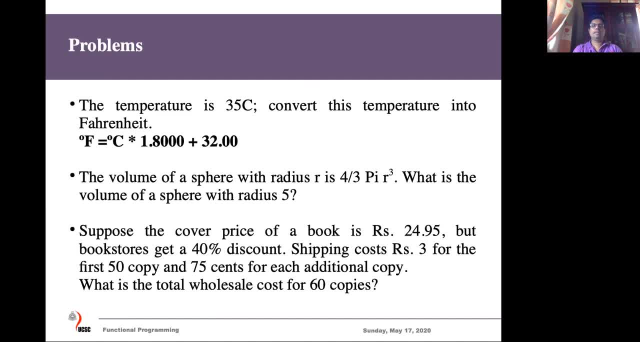 Activities or whatever As the name of the repository. And whatever you do, program Should push to the JIT And you have to then submit the Link of the repository As a submission. So I will Check the link And the time you push. 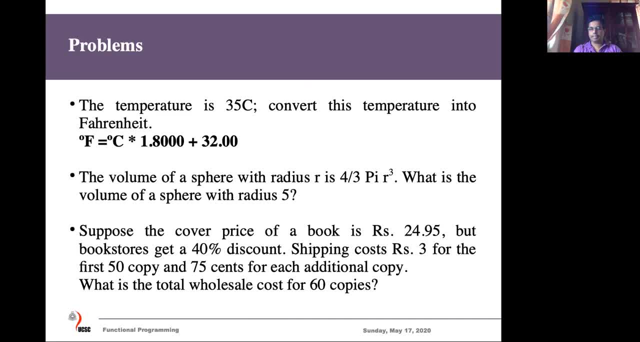 Your course to the link While marking Assignments. So the course should push- Always push to the repository. I am checking the repositories. Each assignment You have to upload Your repository name As the submission. But I will check. 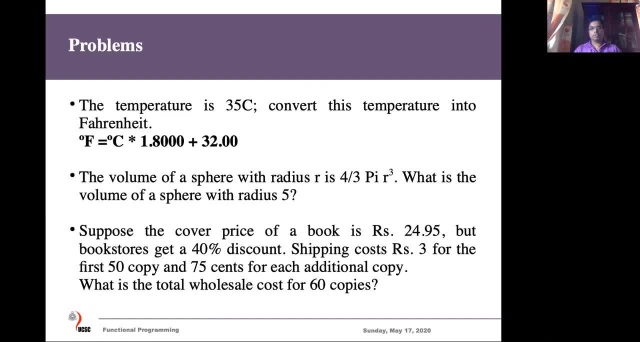 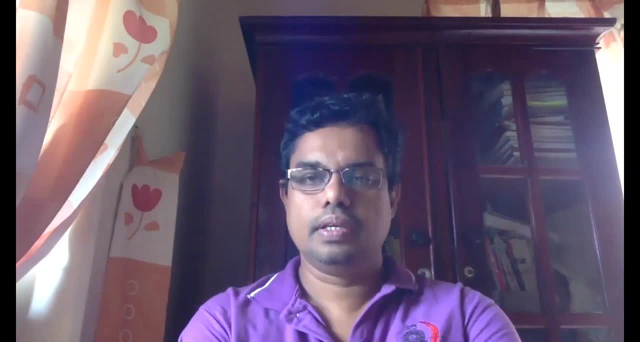 Actually the date of uploading. You are pushing the course To the repository While marking, So that's how we should Continue on Learning in this course. That's it For today, Thank you.